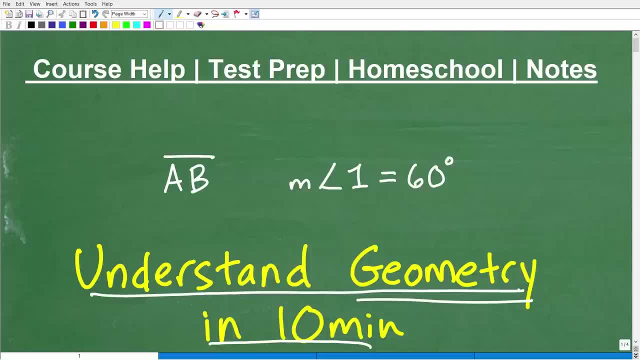 I'm going to leave a link to my math help program in the description of this video, along with my geometry course. Okay, direct link to my geometry course. So if you are taking geometry, you can just go directly there to check out my course. It's very, very, very comprehensive and will definitely help you out. But if you are struggling in mathematics- whether it be geometry, algebra, any other course- I can help you out. I've been teaching math for decades And one of the things I like to think of myself as doing when it comes to mathematics is: 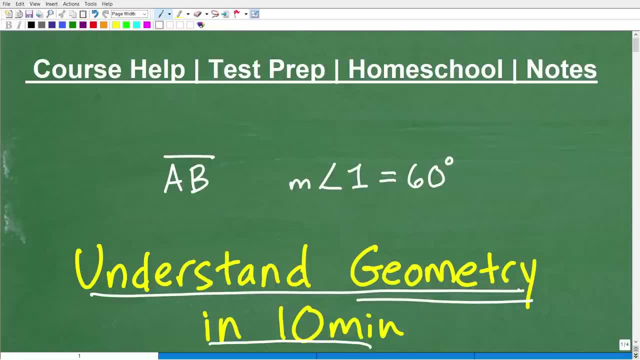 really explaining it versus teaching it. I really break things down in super clear and understandable bite-sized pieces so anyone can get this stuff. So if you're at the middle school, high school or college level, I can definitely help you out. Now, if you happen to be preparing, 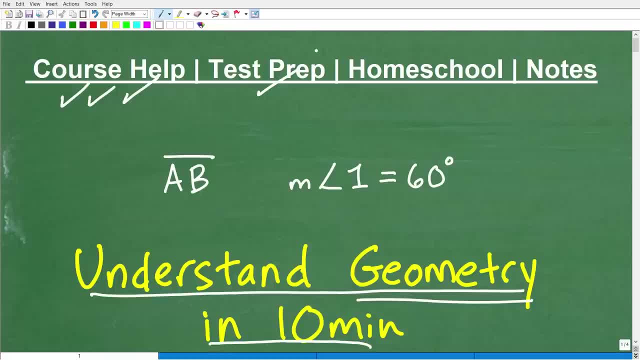 for some test that has a math section on it. I'm talking about things like the GED, SAT, ACT, GRE, GMAT, ASVAB, ACUPLACER, CLEP exam, maybe a teacher certification exam. 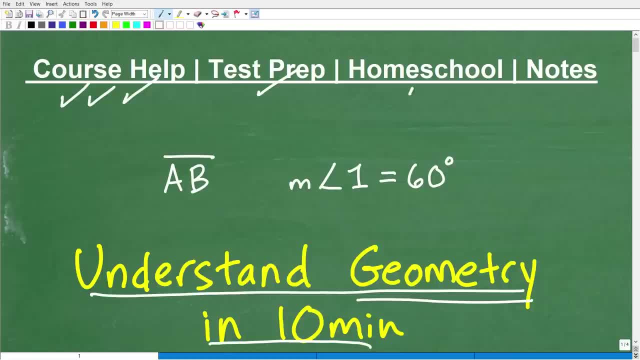 I can definitely help you out And if you homeschool, check out my homeschool math courses. We were just voted number one in the area of middle and high school math. We're pretty proud of that award. We're going to- actually this was from a big 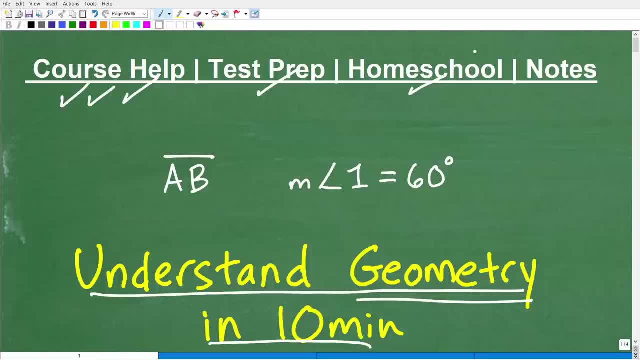 national publication. We're going to be given more information on that very, very soon. Now, if you don't have any math notes, you need to start taking excellent math notes. That's the only way you're going to get great grades in math. But in the meantime, I'm going to leave links to my math. 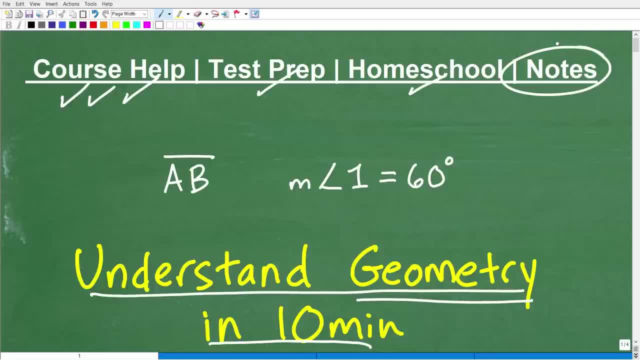 notes so you can check those out. You'll find them in the description of this video as well. Okay, so let's get into high school level geometry And we're going to take a look at the chapters of my course which are, effectively- this is pretty similar to what you would find in any other kind- 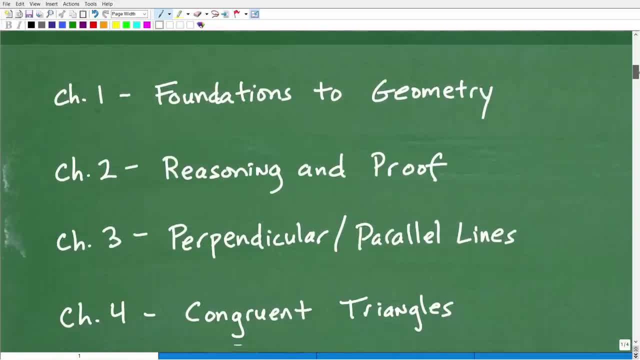 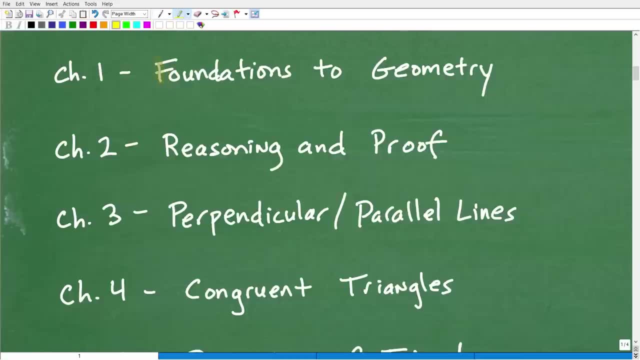 of geometry course, but we're going to walk through them one at a time. Okay, I'm going to try to do this in about 10 minutes. We'll see how I do here in a second. All right, so the first chapter. 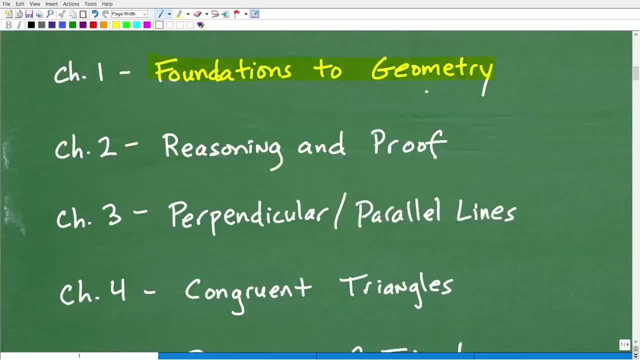 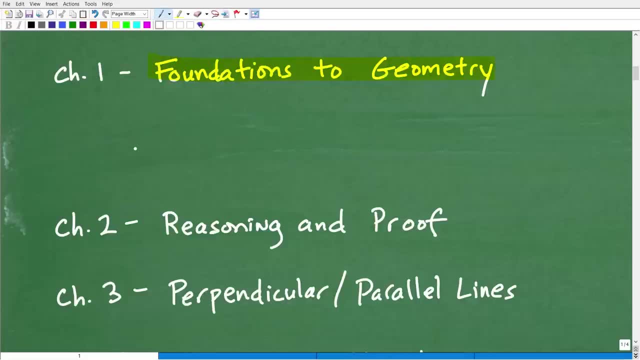 of a geometry course. it's going to be something like this: These are my chapters, by the way, So this would be like the foundations to geometry. So what do you learn in that? Well, you learn things like: hey, what is? 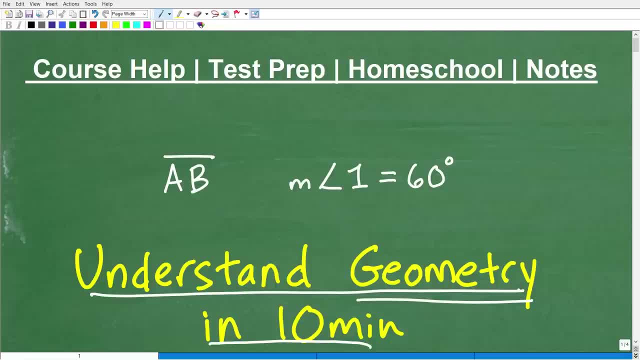 really explaining it versus teaching it. I really break things down and super clear and understandable, bite sized pieces so anyone can get this stuff. So if you're at the middle school, high school or college level, I can definitely help you out. Now, if you happen to be preparing for some test that has a math section on it- I'm talking about things like the GED, SAT, ACT, GRE, GMAT, ASVAB, ACUPLACER, CLEP exam, maybe a teacher certification exam- I can definitely help you out. And if you homeschool, you absolutely. 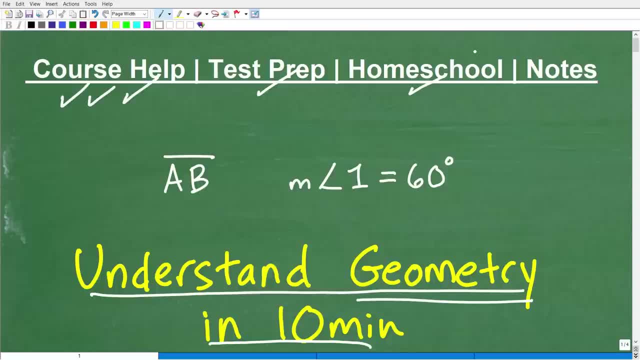 must check out my homeschool math courses. We were just voted number one in the area of middle and high school math. We're pretty proud of that award. We're going to- actually, this was from a big national publication. We're going to be given more information on that very, very soon. Now, if you don't have any math notes, you need to start taking excellent math notes. That's the only way you're going to get great grades in math. But in the meantime, I'm going to leave links to my math notes so you can check those out. You'll find them in the description of this video as well. 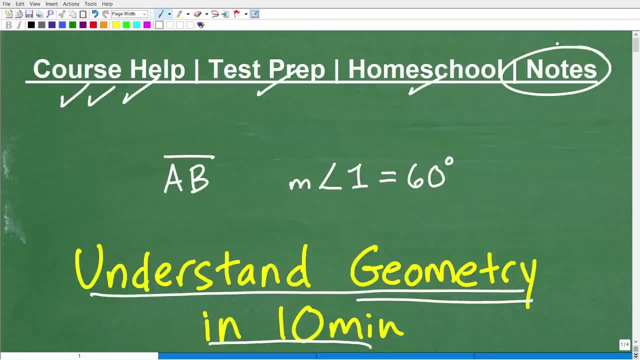 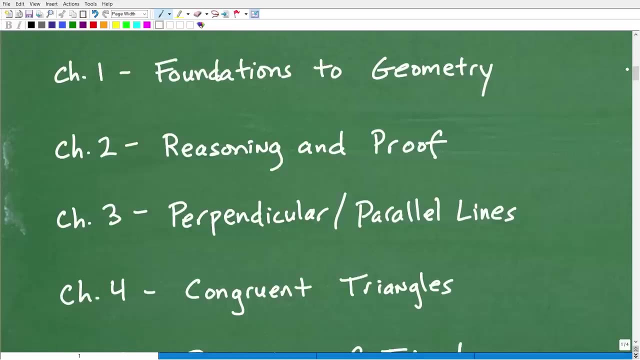 Okay, so let's get into high school level geometry And we're going to take a look at the chapters of my course, which are effectively- this is pretty similar to what you would find in any other kind of geometry course, but we're going to walk through them one at a time. Okay, I'm going to try to do this in about 10 minutes. We'll see how I do here in a second. All right, so the first chapter of a geometry course is going to be something like this. These are my chapters, by the way, So this would be like the foundations to geometry. 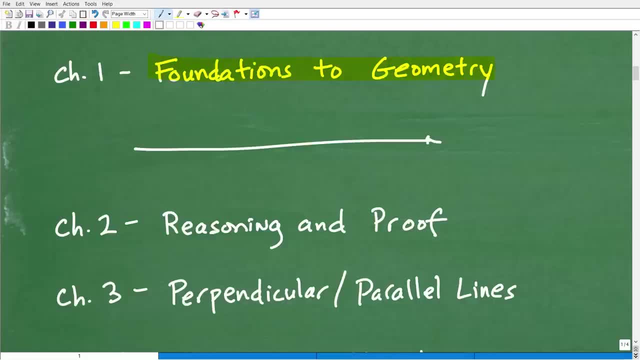 So what do you learn in that? Well, you learn things like: hey, what is a line, What is a point? You learn terms like collinear, coplanar, and you learn like basic notation, like like right here, let me just draw something. So if we have this right here would be like a line segment, And then we have endpoints like here's A and there's B, So we could represent this line segment as the notation A- B. Then we learn how to write angles. So if we have like 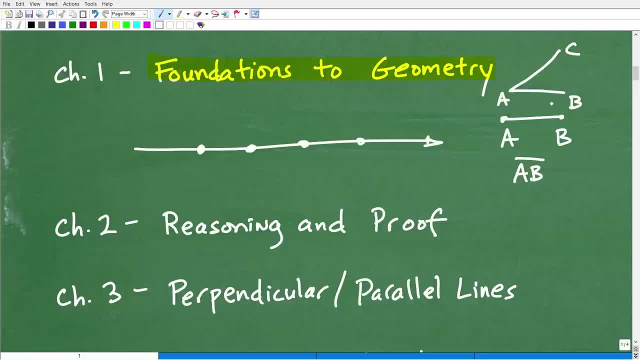 like A B C. This would be like angle B A C. Okay, the A here is in the center, So this goes B A C or C A B, So this would be angle B A C. So in foundations to geometry, just learn some. 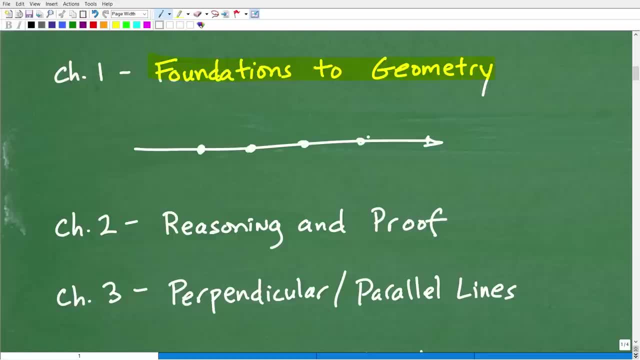 a line, What is a point? You learn terms like collinear, coplanar, and you learn like basic notation, like right here, Let me just draw something. So if we have this right here would be like a line segment, And then we have endpoints like here's A and there's B, So we could represent. 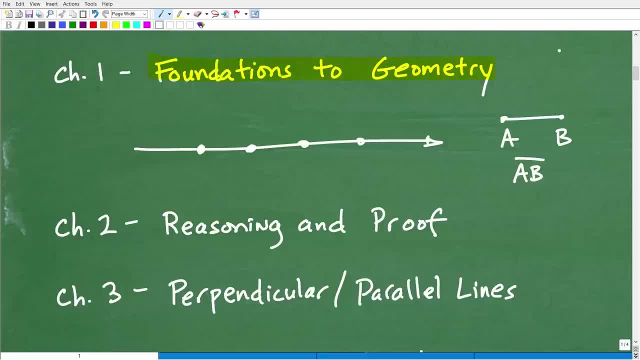 as the notation AB. Then we learn how to write angles. So if we have like ABC, this would be like angle BAC. Okay, the A here is in the center, So this goes BAC or CAB, So this would be angle BAC. 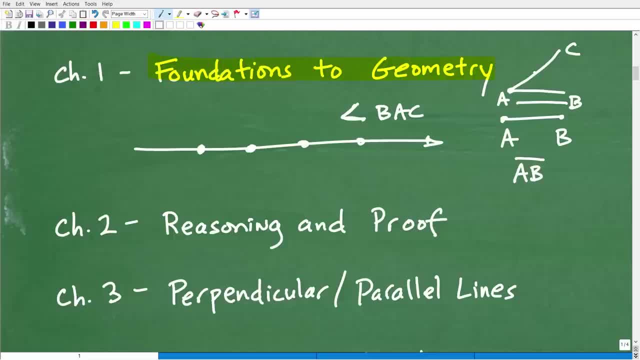 So in foundations to geometry just learn some basic definitions about what points are, what a plane is and angles and some other basic type stuff. So it's not too difficult, just a lot of kind of introductory level type of information. All right, let's move on to chapter two. 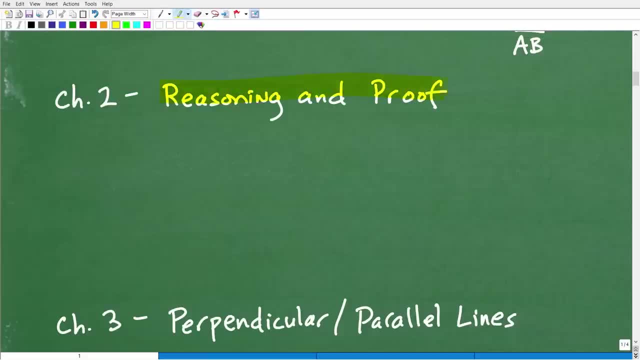 Now, one of the big things in high school geometry is doing proofs, And typically students look like this when they do proofs. They just don't like proofs. They're just like: no, anything but proofs. That's so scary. Listen, if you have taken geometry or taken it. 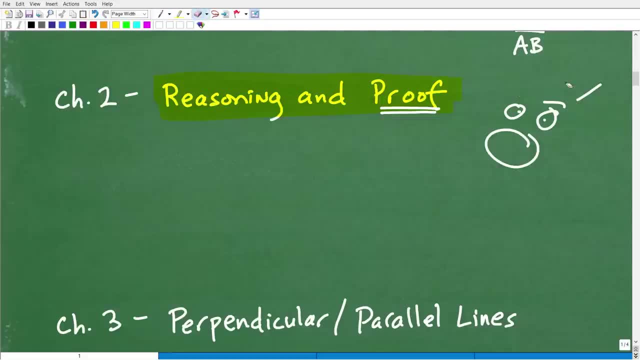 you can understand what I'm talking about. But a proof is you have to prove something, And this is a pretty big deal. Okay, so, reasoning and proof. this has to do with things like logic And it's real. in high school level geometry, you deal with things called. 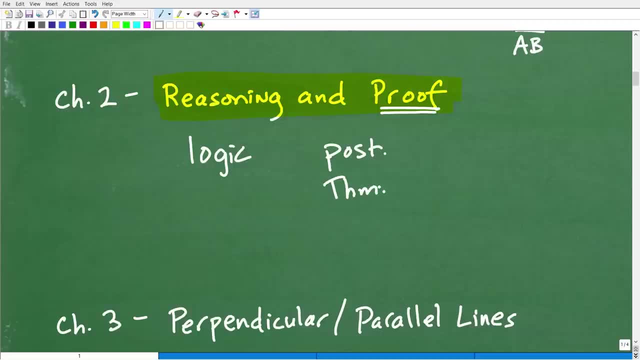 postulates- okay, and theorems- You're going to learn the difference, But you're also going to learn about logic, and specifically deductive logic- okay, and how to construct a geometric proof- All right, this is a pretty big deal, And you're going to learn how to construct a geometricnya. 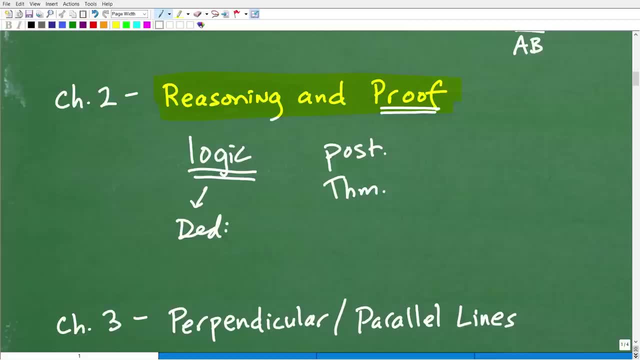 All right, so that's what I'm talking about. But if you're not familiar with geometry, you're going to very, very important. and again, most students are a little bit thrown off by this because they never really kind of studied logic before in any kind of 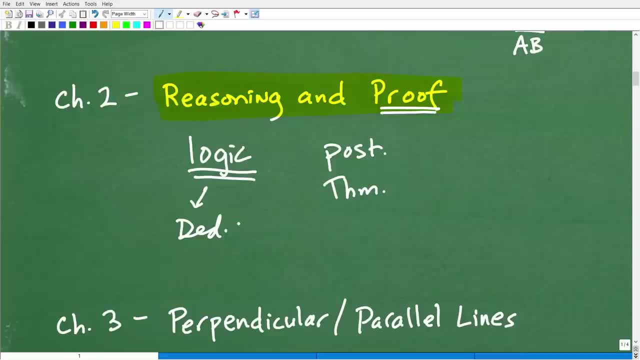 formal sense, but this is very, very important stuff. so, in geometry, in a high school, of a geometry course, some of the questions- not all the questions, obviously, but you're going to see proof questions which are going to be like: prove something. okay, this situation, you're going to have to construct a. 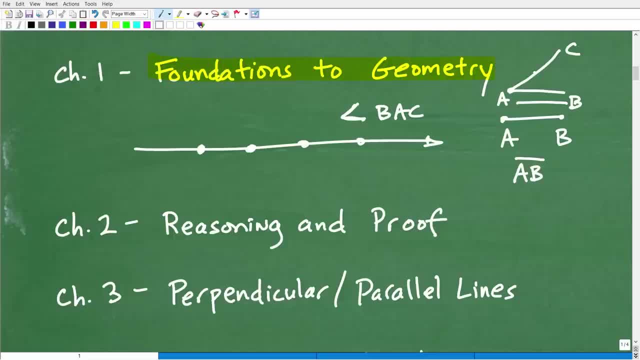 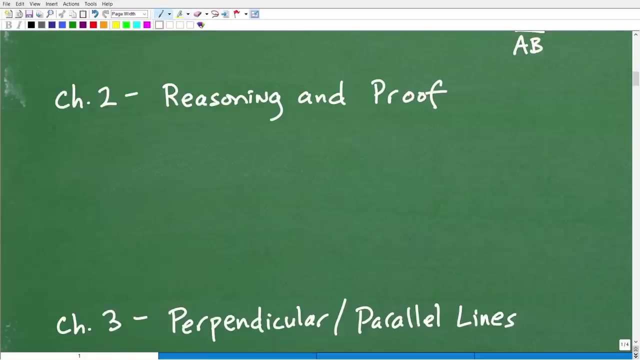 basic definitions about what points are, what a plane is, how to represent angles and some other basic type stuff. So it's not too difficult, just a lot of kind of introductory level type of information. All right, let's move on to chapter two. Now one of the big things in high school. 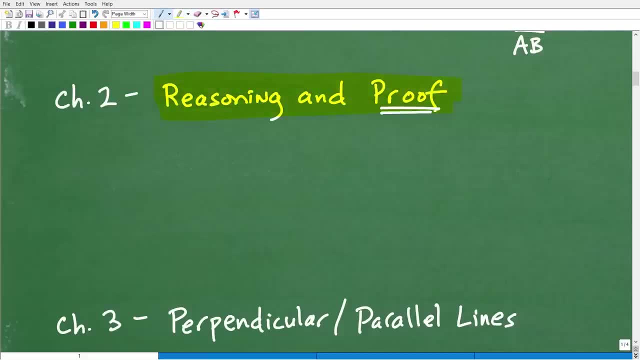 geometry is doing proofs And typically students look like this when they do proofs: They just don't like proofs, They're just like: no, anything but proofs. That's so scary. Listen, if you have taken geometry or taken it, you can understand that. So you can understand that. So you can. 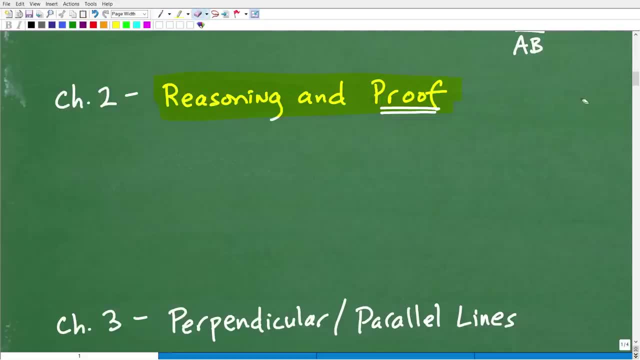 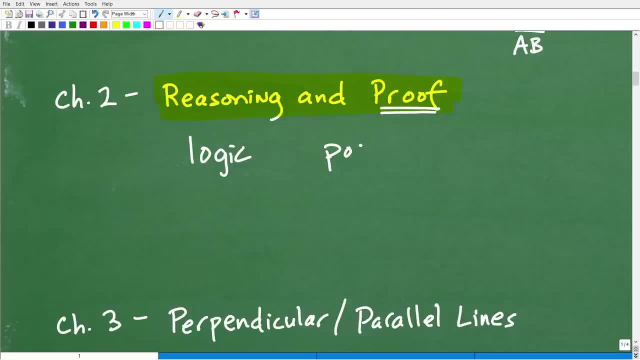 In high school level geometry, you deal with things called postulates- Okay- and theorems. you're going to learn the difference, But you're also going to learn about logic, and specifically deductive logic- Okay, And how to construct a geometric proof- All right. this is very, very. 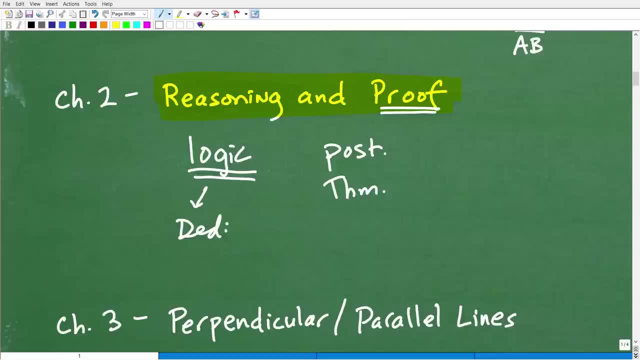 important. And again, most students are a little bit thrown off by this because they never really kind of studied logic before in any kind of formal sense. But this is very, very important stuff. So in geometry, in a high school level geometry course, some of the questions, not all the 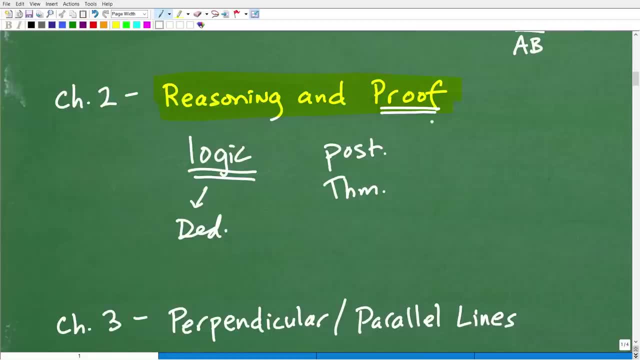 questions, obviously, but you're going to see proof questions which are going to be like: prove something. Okay, this situation: you're going to have to prove something And you're going to have to construct a proof, And a lot of students find this very difficult. So, anyways, you're going to 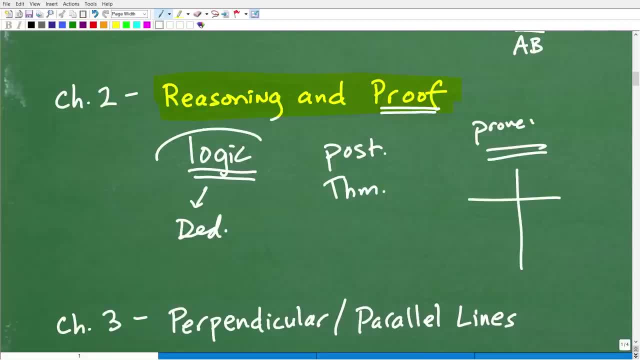 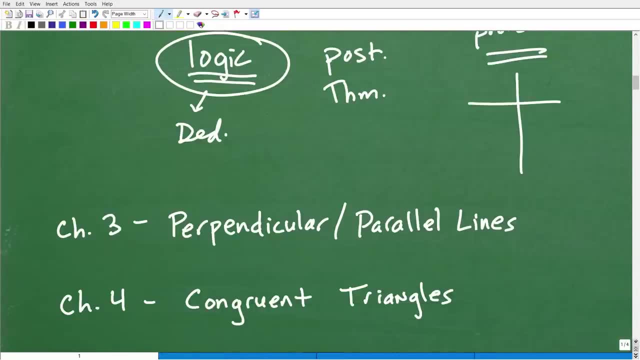 encounter this, But again, really, you're going to be learning about logic, Okay, which is very interesting, by the way, as well, So I think a lot of you actually might enjoy that. All right, let's move on to chapter three. By the way, we're looking at 11 chapters in my course. 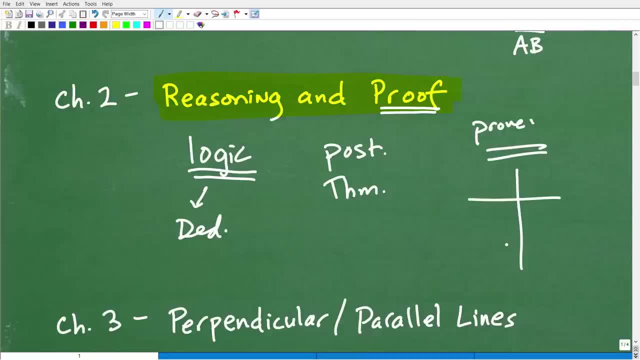 proof, and a lot of students find this very difficult. so, anyways, you're going to encounter this, but again, really, you're going to be learning about a logic okay, which is very interesting, by the way, as well, so I think a lot of you actually might enjoy that. all right, let's move on to chapter 3. by the way, 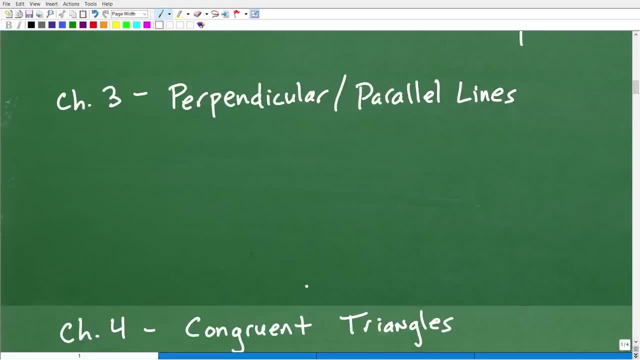 we're looking at 11 chapters in my course, so chapter 3 is going to be in my course. it's a perpendicular and parallel lines. okay, so what are parallel lines? well, parallel lines are lines that never cross one another. so here is L and here is M. we 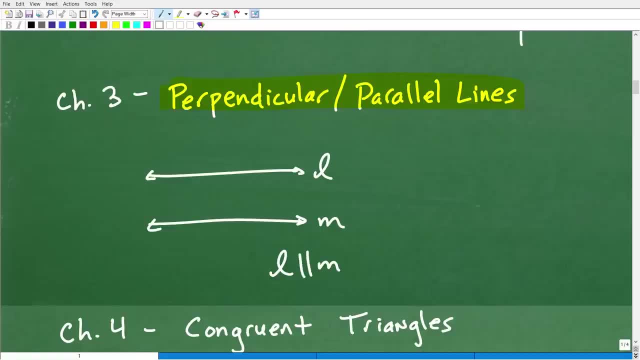 can say: L is parallel to M. and what are perpendicular lines? well, we have line L here and then we have another line right there, M, and these two lines are perpendicular. so there's a heavy emphasis on parallel lines and all the angles that are created when you have two parallel lines and something called a transversal 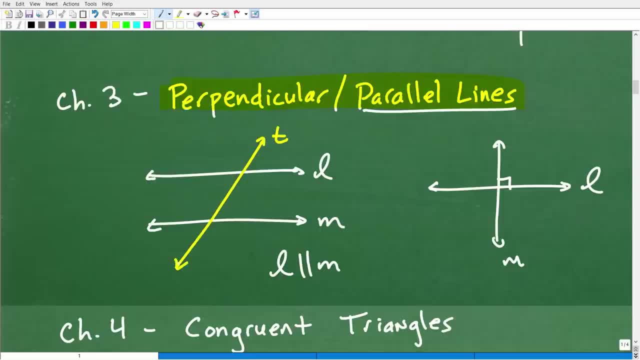 that chops through them. okay, so when you have a transversal, which is another line that chops through two parallel lines, all kinds of angles are created. you got these things called vertical angles. you got all alternate interior angles, same side interior corresponding angles. so you're really going to study this pretty. 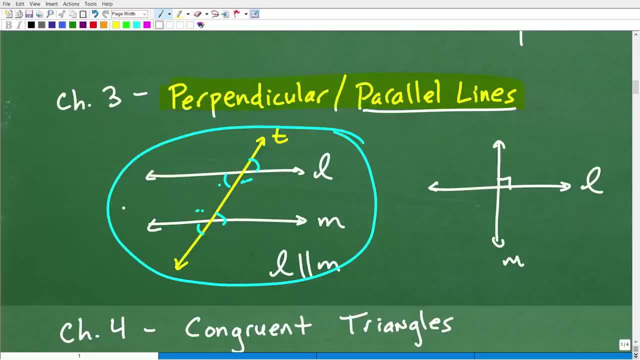 heavy-duty and, by the way, I must say that a lot of the problems are going to be a little bit more catastrophic than what we're doing with this subject. excuse me, a parallel lines, or perpendicular lines in the way, is going to require you to know some algebra, in case you're going to need to have your algebra skills ready to. 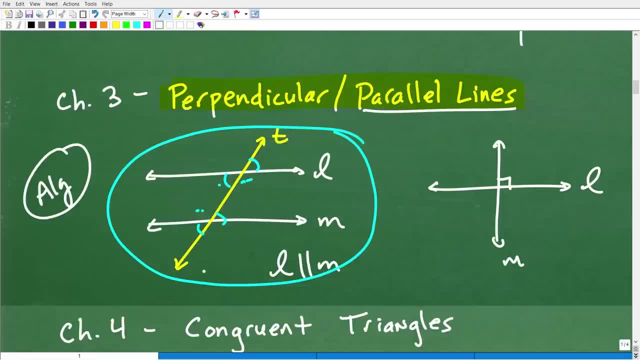 go, but this is a full chapter for any geometry course. so you're going to learn all the different special angles formed when you have a transversal that chops there two or more parallel lines, and then you're going to study more properties and theorems about quarters. please stop. check out my different videos for tutorials. and two or more parallel Used For Pletsch: Important Tutorial. 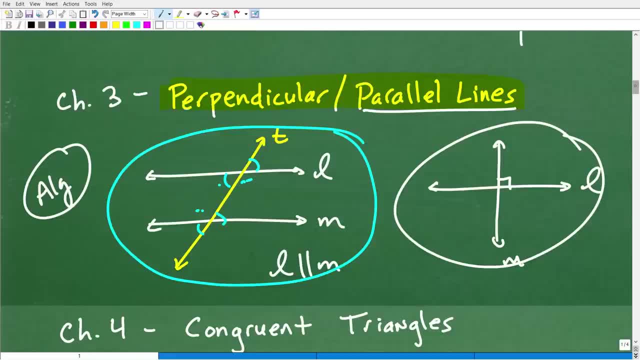 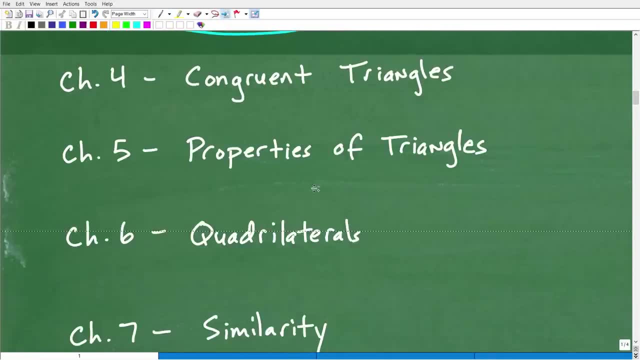 as well. very, very important chapter indeed. okay, let's take a look at chapter four again. each geometry course, every geometry course out there, is gonna have them trying to scoot this down. that's not working. let me see if I could just move this down this way. that'll work okay. so I'm congruent. let's talk about. 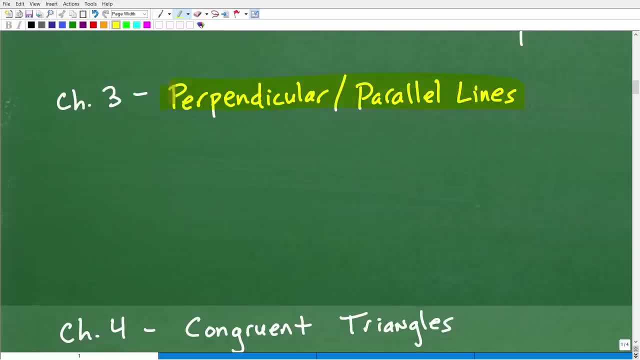 So chapter three is going to be in my course it's perpendicular and parallel lines. Okay, so what are parallel lines? Well, parallel lines are lines that never cross one another. So here is L and here is M. we can say: L is parallel to M. And what are perpendicular lines? Well, we have. 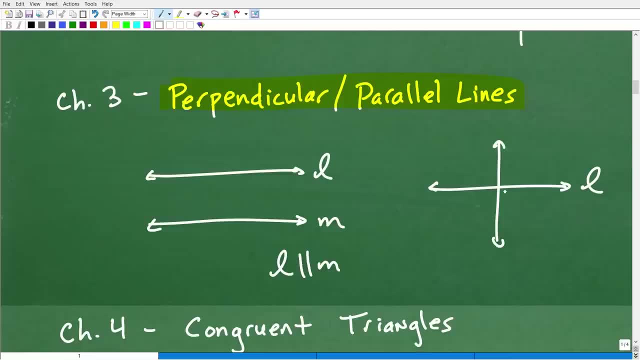 line L here, And then we have another line right there, M, And these two lines are perpendicular. So there's a heavy emphasis on parallel lines and all the angles that are created When you have two parallel lines and something called a transversal. 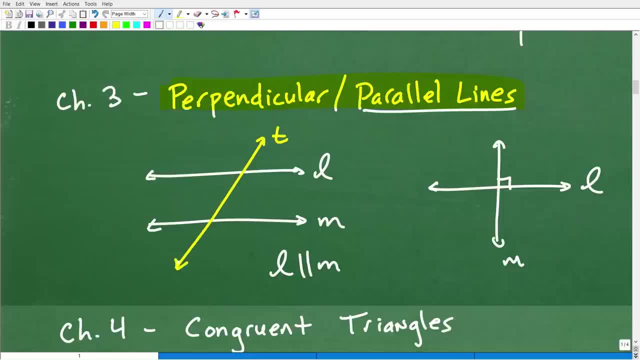 that chops through them. Okay, so when you have a transversal, which is another line that chops through two parallel lines, all kinds of angles are created. You got these things called vertical angles. you got alternate interior angles, same side interior corresponding angles. 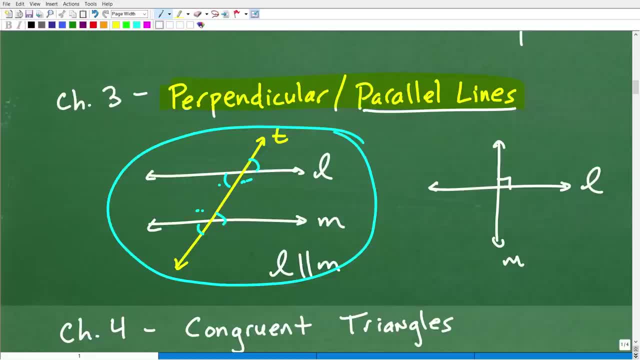 So you're really going to study this pretty heavy duty And, by the way, I must say that a lot of the problems you're going to be doing with this subject- excuse me, parallel lines or linear lines- is going to require you to know some algebra. Okay, so you're going to need to have 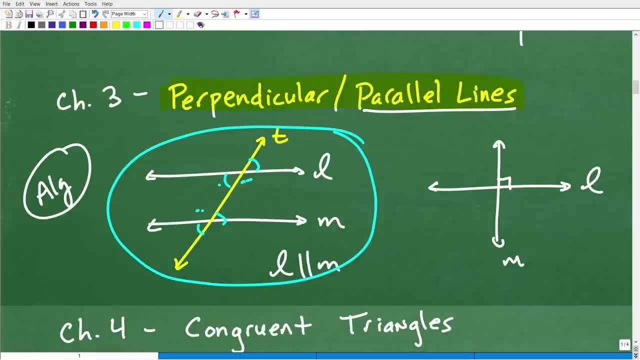 your algebra skills ready to go, But this is a full chapter for any geometry course, So you're going to learn all the different special angles formed when you have a transversal that chops through two or more parallel lines, And then you're going to study more properties and theorems. 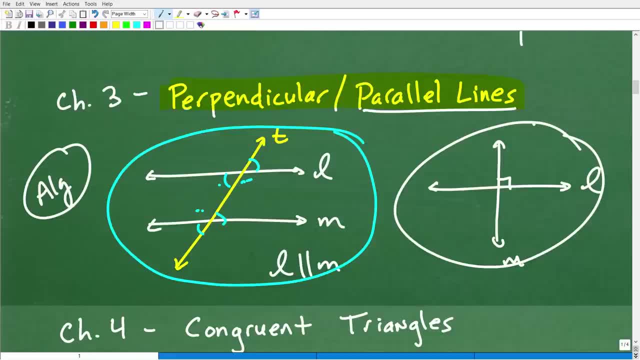 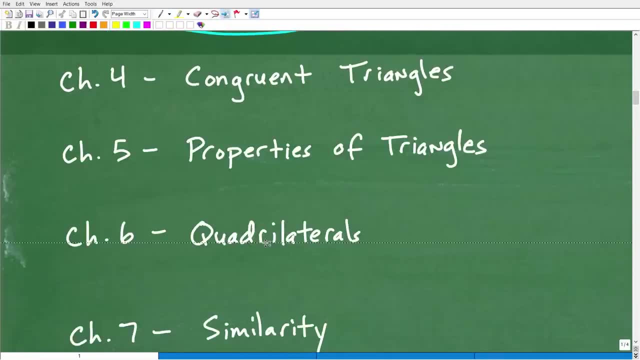 about parallel lines as well. Very, very important chapter indeed. Okay, let's take a look at chapter four. Again, each geometry course, every geometry course out there is going to have. I'm trying to scoot this down, That's not working. Let me see if I can just move this down this way. 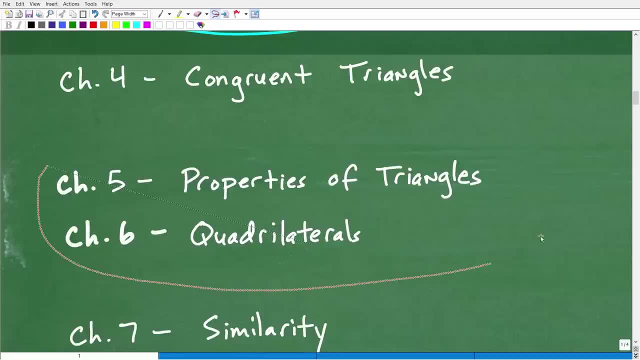 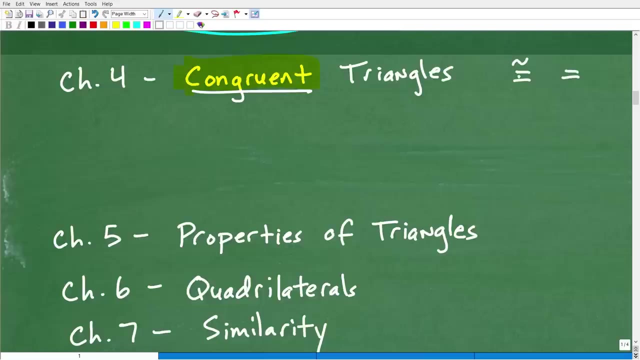 That'll work, Okay, so congruent, Let's talk about congruent triangles. Let me give myself some room, All right. so what does this word right here mean? Well, you need to know this. congruent is this little symbol right there. Okay, so you have equals, this congruent, and. 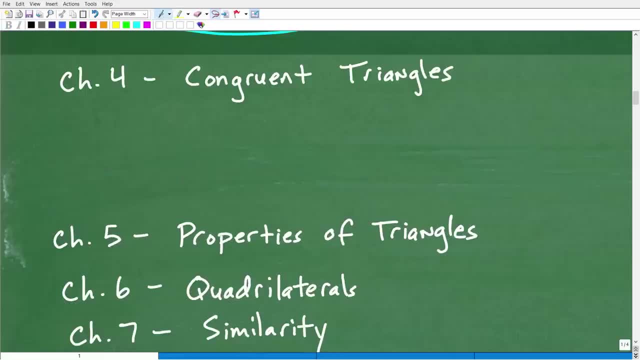 congruent triangles. let me give myself some room, all right. so what does this word right here mean? well, you need to know this from congruent. is this little symbol right there? okay, so you have equals, this congruent. and then this little squealing line is similar. we'll talk about that in a second, so we're. 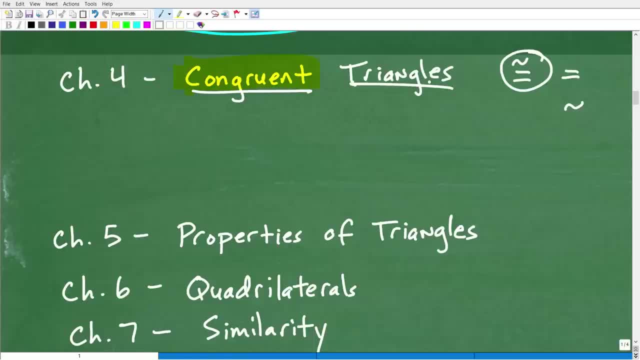 talking about congruency and we're talking specifically about triangles. but congruent triangles mean the exact same size and shape, okay. so if I have a triangle right here, okay, and let's call this a, b, c, and i have the exact same size and shape, let's call this d e, f, so i can write this this way. 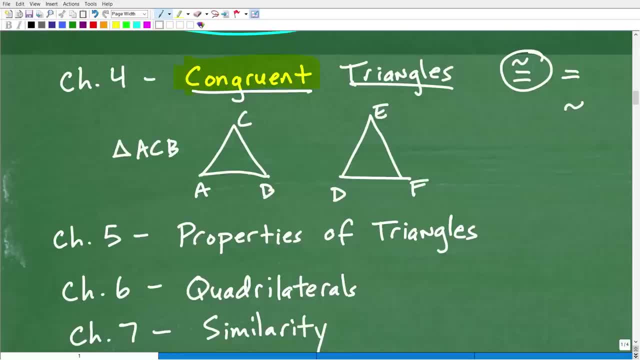 triangle a, c, b and triangle d, e, f. i can say these two triangles are congruent if they have the same angles and same uh sought. the sides are this are the same same length and the angles are the same. in other words, they're exact copies of one another. that's what you have to understand. 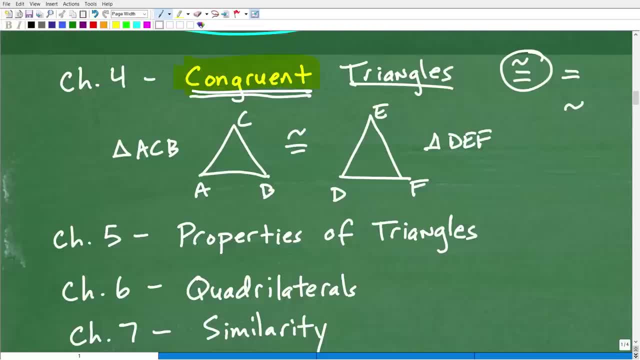 about congruency. it's basically an exact copy of a figure. okay, now, of course, in this particular chapter, you're going to be talking about congruent triangles and you're going to be learning all kinds of postulates and theorems, things like uh s s s, side, side, side. so if you have two triangles, 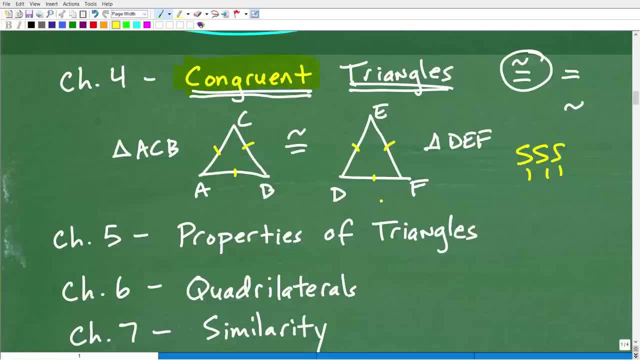 and each of the sides are the same lengths, you um have congruent triangles. okay, so you're going to be learning some, uh, various theorems and postulates that uh, in order for you to be able to prove, and this is where that idea of proof is going to come. 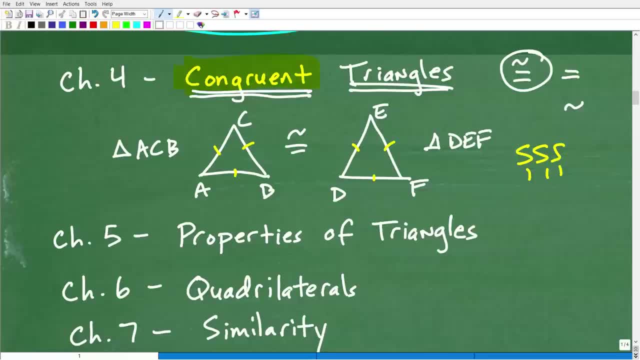 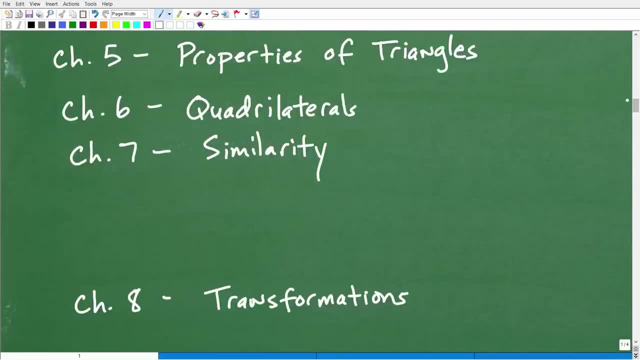 in that you you can prove that you have two triangles are congruent. okay, so congruency is a big deal in geometry. all right, let's move down to our next chapter and notice we are talking about: um. no, i can't really scroll down here. it's not working for me too well, but i'm just going to. 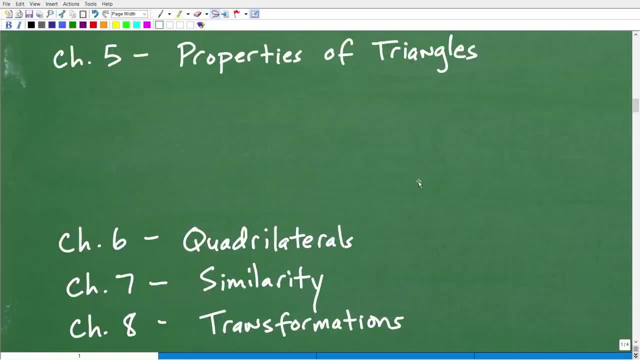 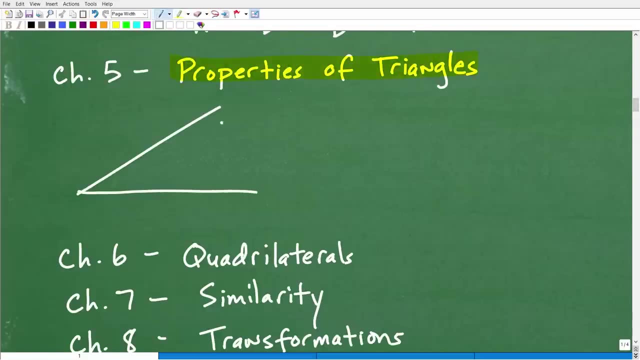 move things down this way. okay, so we're going to be, um, talking about, uh, properties of triangles. okay, so what are we talking about there? well, you're going to be really looking at triangles in depth. you're going to talk about angle bisector theorems. so, if i have an angle right here in a 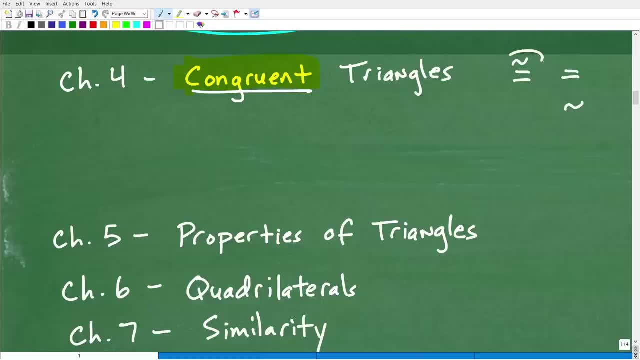 this little squiggly line is similar. We'll talk about that in a second. So we're talking about congruency And we're talking specifically about triangles. but congruent triangles mean the exact same size and shape, Okay. so if I have a triangle right here, okay, and let's call this ABC, And I 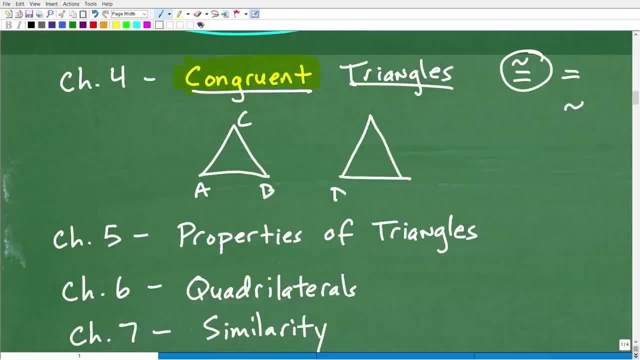 have the exact same size and shape. Let's call this D E F. So I can write this this way: triangle C B and triangle D E F. I can say these two triangles are congruent if they have the same angles and same sought. the sides of this are the same same length and the angles are the same. 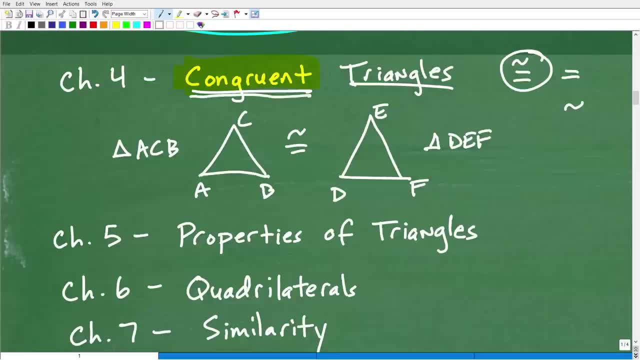 In other words, they're exact copies of one another. That's what you have to understand about congruency. It's basically an exact copy of a figure. Okay, now, of course, in this particular chapter, we're going to be talking about congruency. So we're going to be talking about congruency. 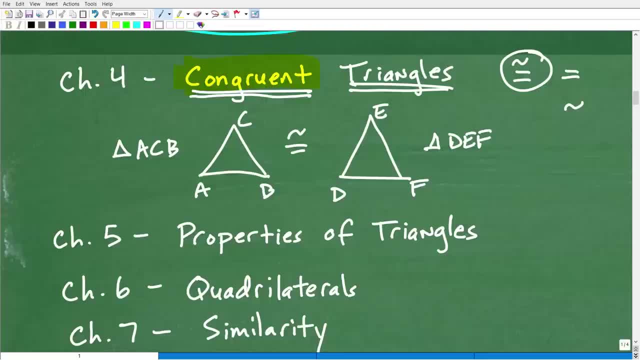 And we're going to be talking about congruent triangles And you're gonna be learning all kinds of postulates and theorems, things like SSS, side, side, side. So if you have two triangles and each of the sides are the same lengths, you have congruent triangles. Okay, so you're going. 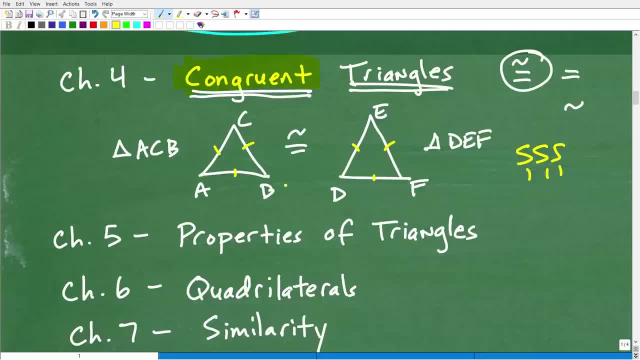 to be learning some various theorems and postulates that in order for you to be able to prove- and this is where the idea of proof is going to come in- that you can prove that you have two triangles are congruent. Okay, so congruency is a big deal in geometry. 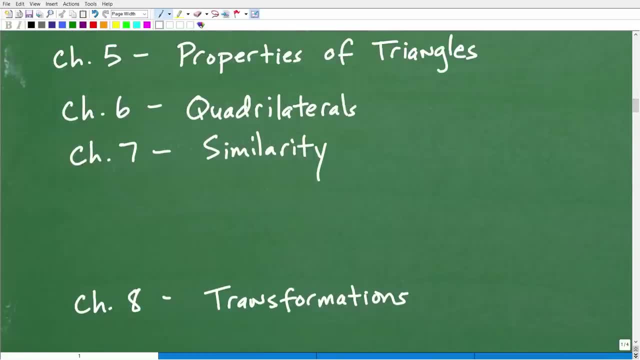 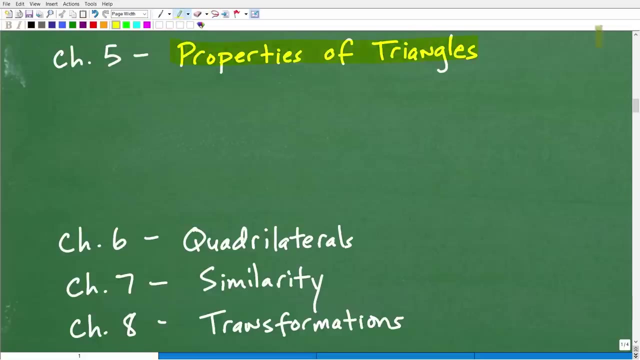 All right, let's move down to our next chapter And notice we are talking about Now. I can't really scroll down here, It's not working for me too well, But I'm just going to move things down this way. Okay, so we're going to be talking about properties of triangles, Okay. 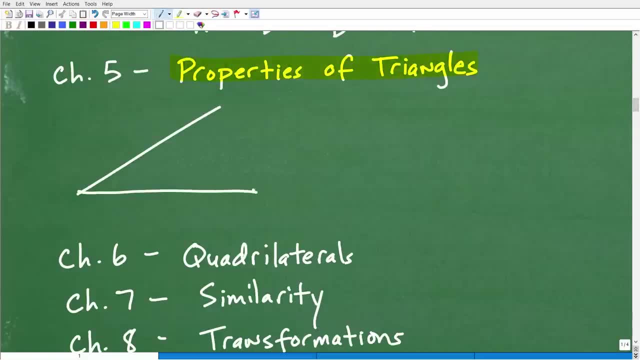 so what are we talking about there? Well, you're going to be really looking at triangles in depth. you're going to talk about angle bisector theorem. So if I have an angle right here and a triangle and I bisect it, in other words, I cut this angle in half, and I cut this angle in half and I cut. 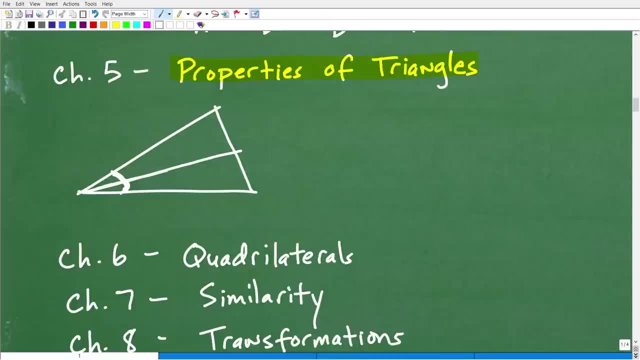 triangle and i bisect it. in other words, i cut this angle in half. what happens to this situation over here? okay, and there's all kinds of theorems and properties. one of the unique things, too, you're going to be learning is about learning about in terms of triangles. is the triangle inequality? 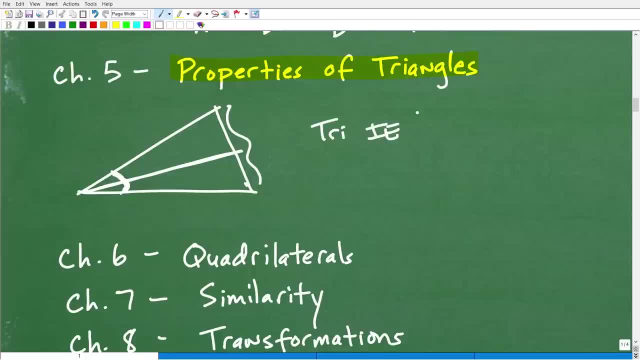 okay, triangle inequality, and i've done a different video on that and i've done a different video on that as well. let's take a look at a triangle inequality problem right now. let me see if i can make something up. so three four five, okay. so this right here: three four five would be the length of 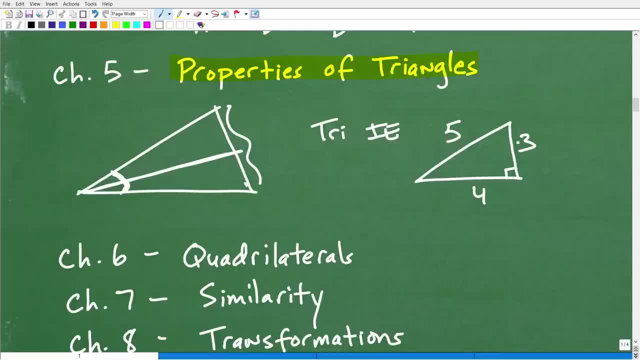 a right triangle. so this is an actual lengths of a triangle. but one of the things about properties of triangles that you're going to study in depth in a geometry course is notice here is that the sum of any two sides is always greater than the third side of a triangle and the sum of any two. 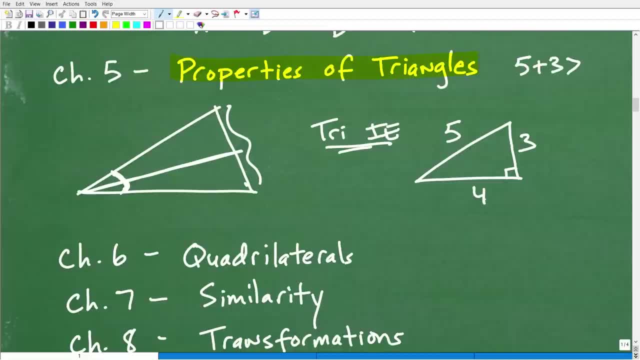 triangles. so, for example, five plus three is going to be greater than four. three plus four is greater than five. excuse me, and uh, let's see. what else are we missing here? uh, five plus four. five plus four is greater than three. so any two sides when you add up in a triangle. 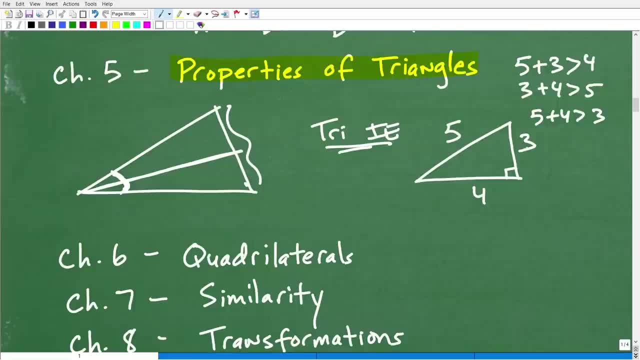 hat must be greater than that third last side remaining, just as i showed you right here. if it isn't, then you, then the lengths given, uh, could not form a triangle. okay, so this is going to be part of the stuff that you're going to be learning, and the properties of triangles again. angle bisector. 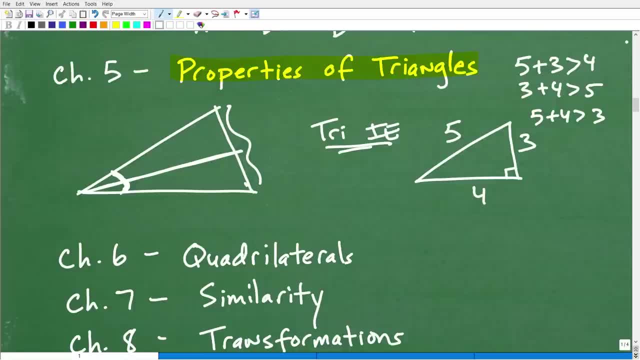 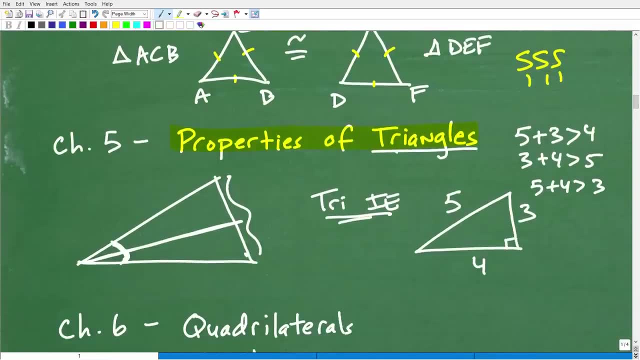 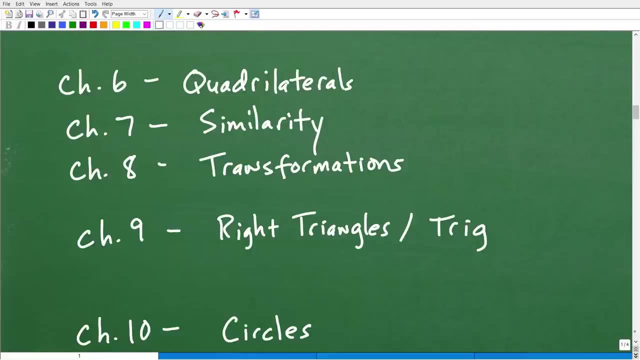 theorems and triangle inequality- very, very important stuff. again, heavy emphasis on triangles. okay, we're talking about congruent triangles and we're talking about, uh, properties of triangles. and we'll actually be studying triangles even further down the road here, in a second i will show you because we'll talk about right triangles. but let's move on to our next chapter. 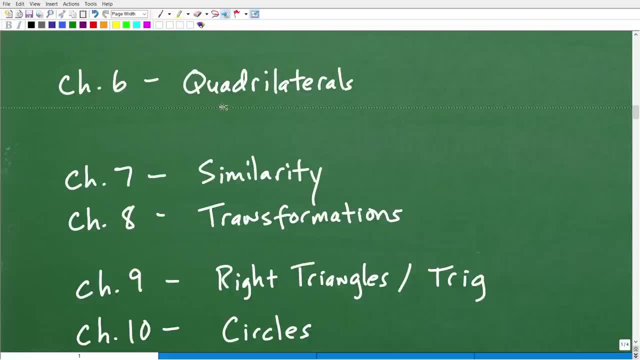 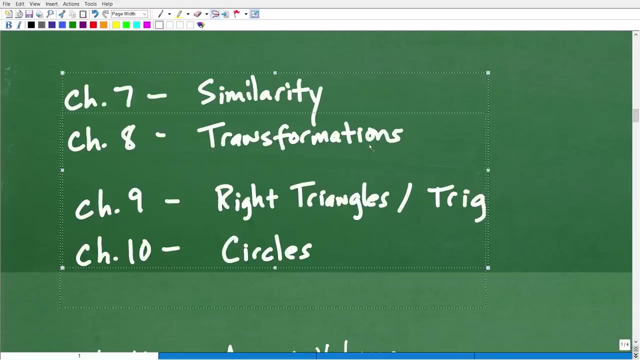 and uh. hopefully i'm doing okay on time. i don't think i'm going to be doing this in 10 minutes, especially with the way my uh thing is going here. normally i'm able to space this out, but let me just fix this real quick. i apologize for any difficult technical difficulties, but we're 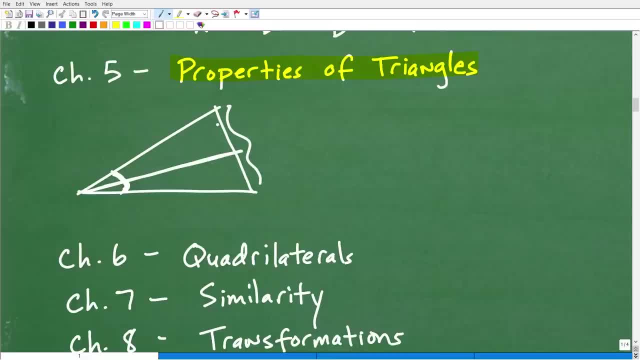 half what happens to this situation over here. okay, there's all kinds of theorems and properties. one of the unique things, too, you're going to be learning is about learning about in terms of triangles. is the triangle inequality? okay, triangle inequality, and i've done different videos on that. 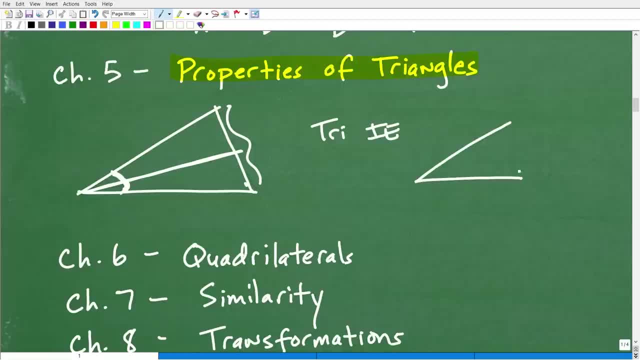 as well. let's take a look at a triangle inequality problem right now. let me see if i can make something up. so three, four, five, okay. so this right here: three, four five would be the length of a right triangle. so this is an actual length of a triangle. but one of the things about properties 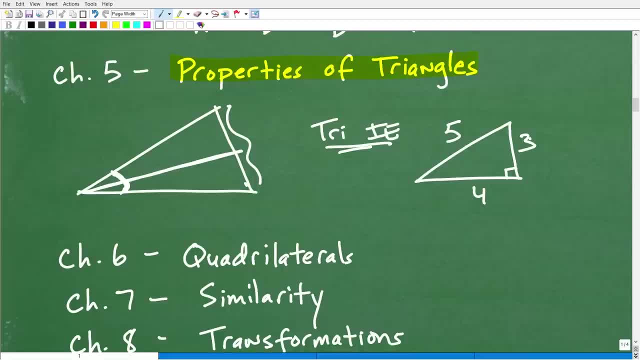 of triangles that you're going to study in depth in a geometry course is. notice here is that the sum of any two sides is always greater than the third side of a triangle. so, for example, five plus three is going to be greater than four, three plus four. 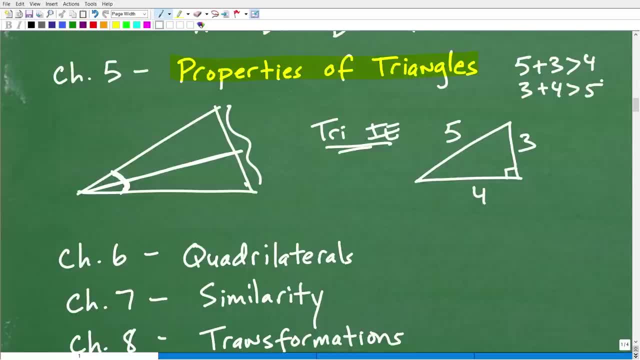 is greater than five. excuse me, and uh, let's see what else are we missing here? uh, five plus four. five plus four is greater than three, so any two sides when you add up in a triangle hat must be greater than that. third, uh, last side remaining, just as i showed you right here. 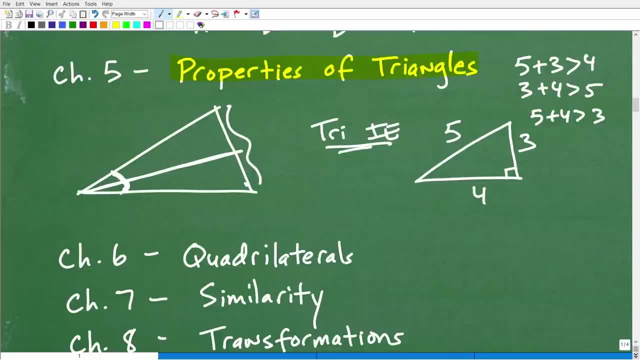 if it isn't, then you, then the lengths given uh could not form a triangle. okay, so this is going to be part of the stuff that you're going to be learning, and the properties of triangles again, angle, bisector theorems and triangle inequality- very, very important stuff. again, heavy emphasis. 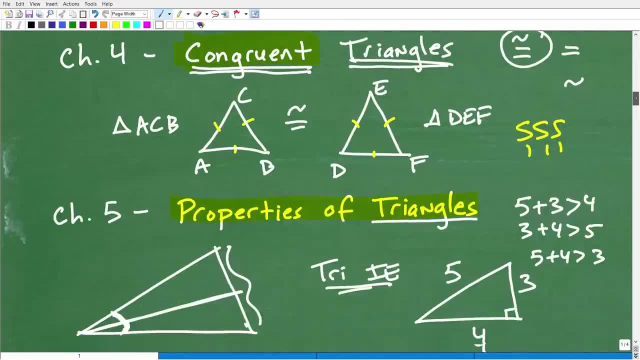 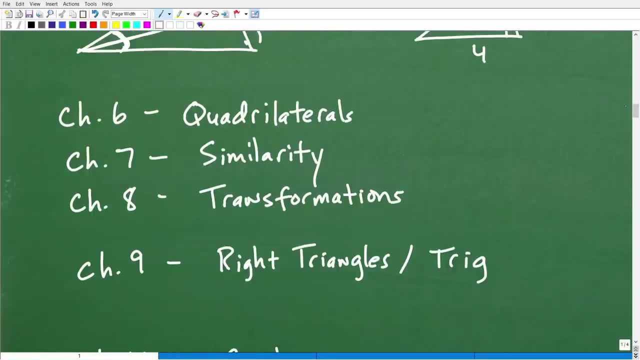 on triangles. okay, we're talking about congruent triangles and we're talking about, uh, properties of triangles. and we'll actually be studying triangles even further down the road here in a second i will show you, because we'll talk about right triangles. but let's move on. 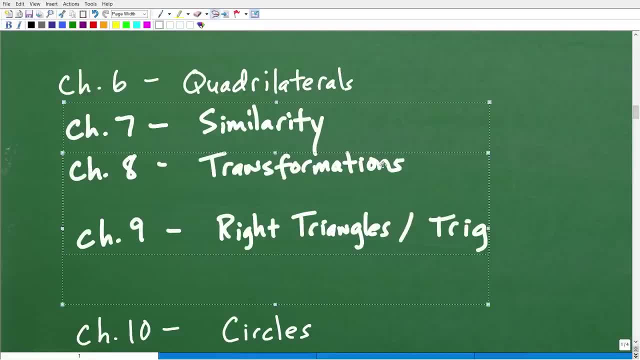 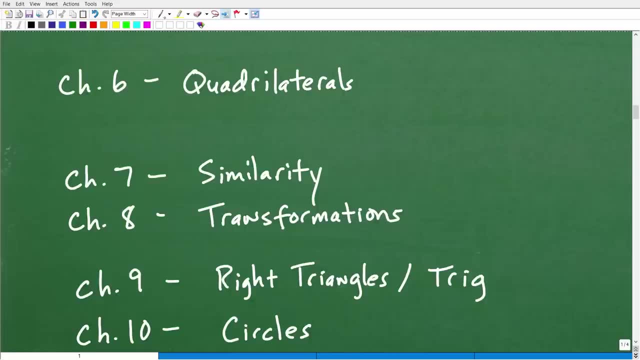 to our next chapter and, uh, hopefully i'm doing okay on time. i don't think i'm going to be doing this in 10 minutes, especially with the way my uh thing is going here. normally i'm able to space this out, but let me just fix this real quick. 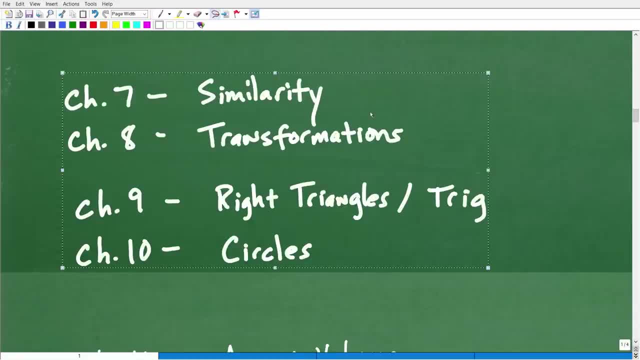 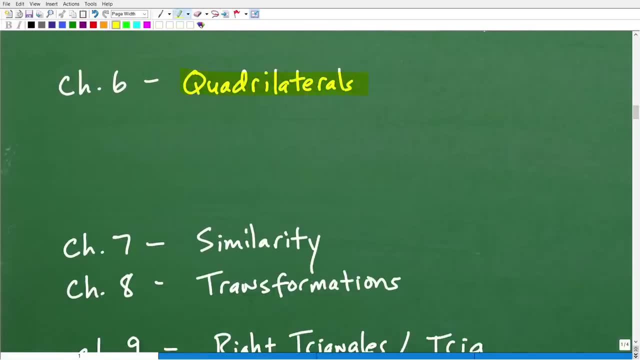 i apologize for any difficult technical difficulties, but we're not going to let that stop us learn some high school geometry here, okay? so let's talk about the next thing here. uh, quadrilaterals, big big word, and um, quadrilaterals are four-sided closed figures, okay, that are constructed with lines, things like this. so what type of quadrilaterals are we talking? 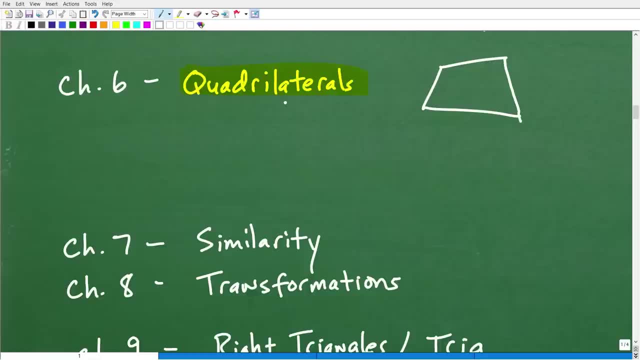 about. well, this is really. quadrilaterals are a type of polygon, okay, so we're talking about a four-sided polygon and you're going to be studying things like the rectangle, all the properties of a rectangle, uh, trapezoid is another one, uh, a rhombus, okay, uh, and a square, all right, so these are you're. 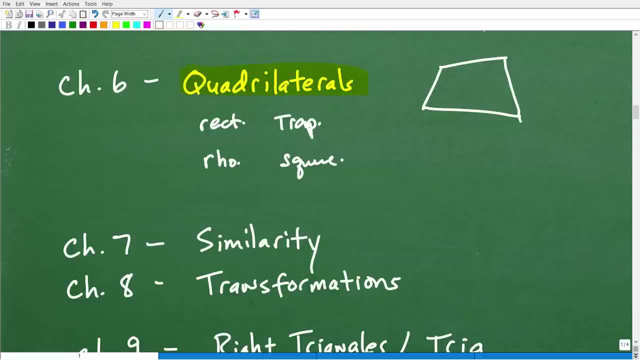 going to be talking about all the different properties with respect to uh quadrilaterals and special quadrilaterals as well. okay, so you're going to have a lot of fun in this particular chapter- very, very important, and now let's move on. oh boy, excuse me right here. 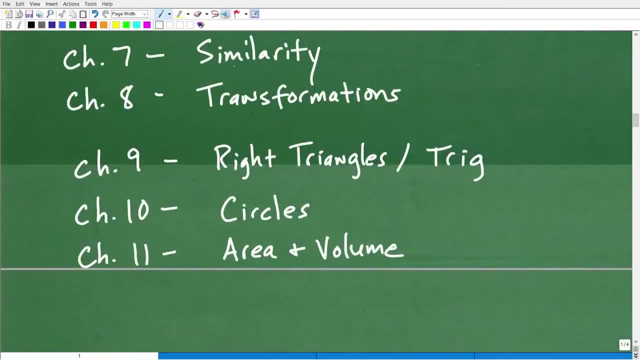 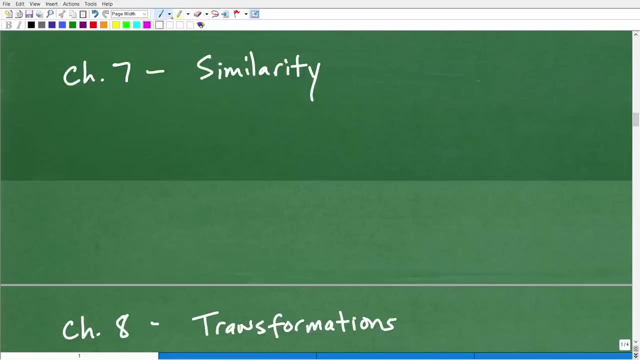 i'm going a little bit too far. let's move on to similarity. okay again, my thing is not working, but i'm not going to stop this video and make this over again. i'm just going to keep plowing away, all right. so let's move on here. similarity- okay. so what is similarity? well, similarity. 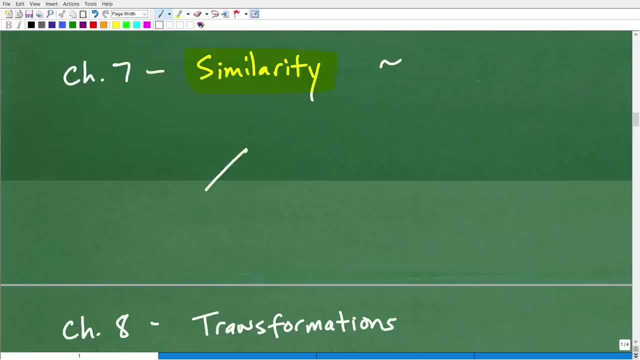 is that one little squiggly figure right there, and i'm going to be talking about that in a little bit there. so let me just kind of show you that. so let's say, i have a little triangle like this, okay, and let's just, uh, kind of really make sure you understand, okay. so these two triangles, 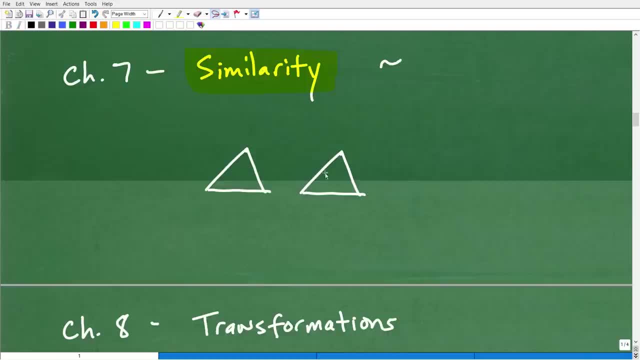 together are exactly the same copy of one another. so these two triangles right here, this would be an example of congruency. that's what congruency or congruency is? it's an exact copy of one another. however, in this particular chapter you're going to be dealing with 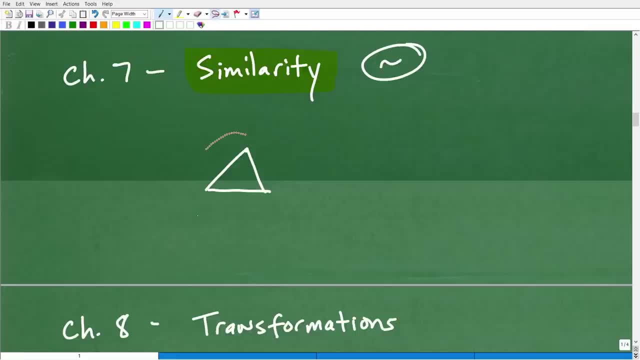 similarities and you're going to be dealing with similarities and you're going to be dealing with similarity. and similarity is a different deal, and similarity is kind of a zoomed in or zoomed out copy of that figure. okay, so if you are given one figure and you zoom in, or if you're given one, 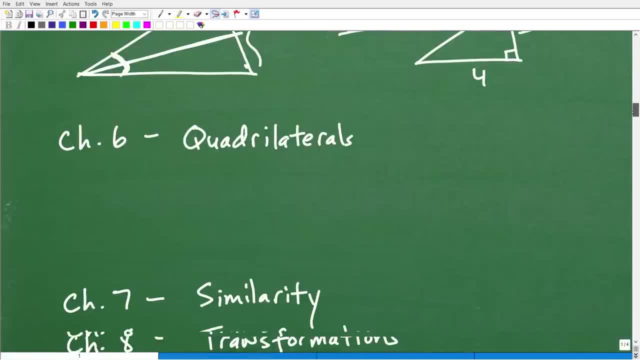 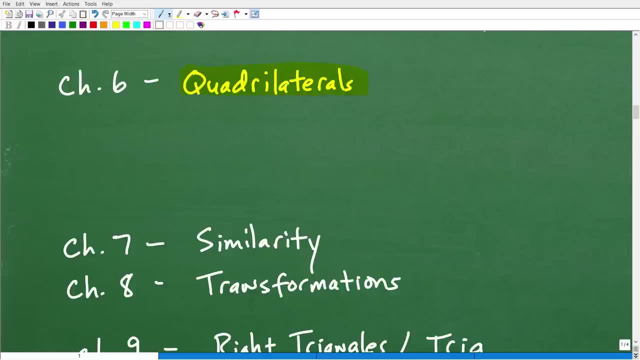 not going to let that stop us learn some high school geometry here, okay, so let's talk about the next thing here. uh, quadrilaterals, big big word, and um. quadrilaterals are four-sided closed figures, okay, that are constructed with lines, things like this. so what type of quadrilaterals are we talking about? well, this is really. quadrilaterals are a. 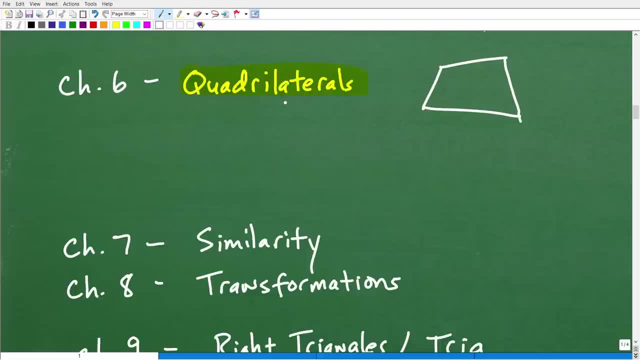 type of polygon, okay, so we're talking about a four-sided polygon, and you're going to be studying things like the rectangle, all the properties of a rectangle, uh, trapezoid is another one, uh, a rhombus, okay, and a square, all right. so these are. you're going to be talking about all the. 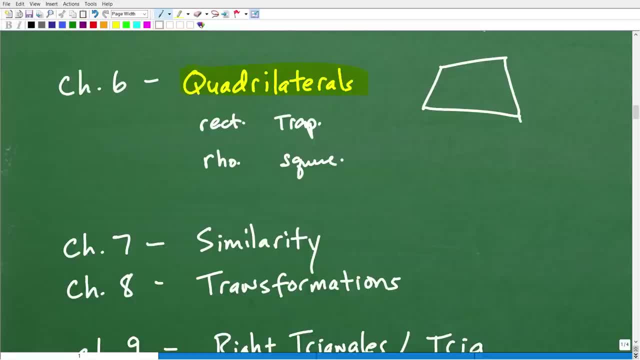 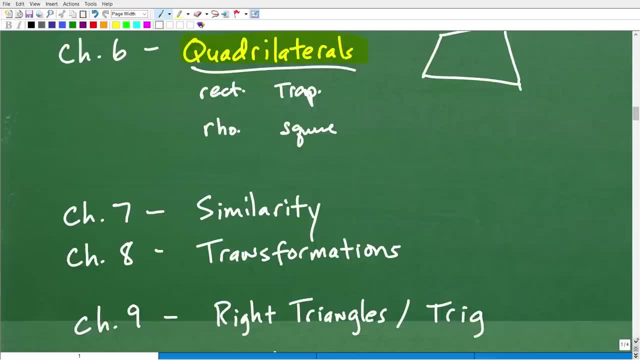 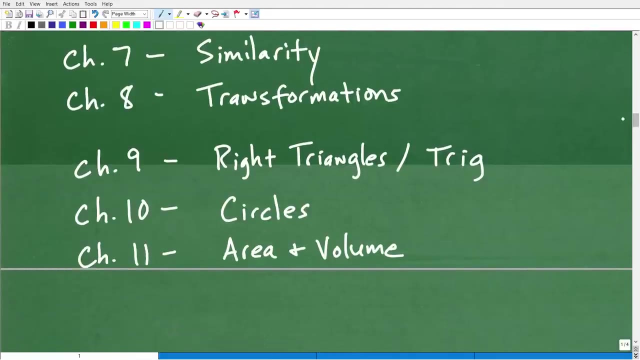 properties with respect to, uh, quadrilaterals and special quadrilaterals as well. okay, so you're going to have a lot of fun in this particular chapter, very, very important. and now let's move on. oh boy, excuse me, right here i'm going a little bit too far. let's move on to similarity. okay, again. 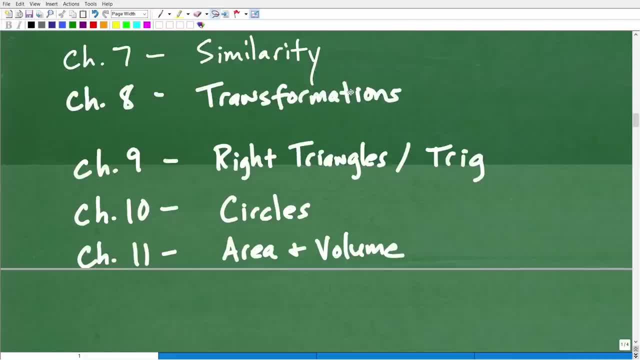 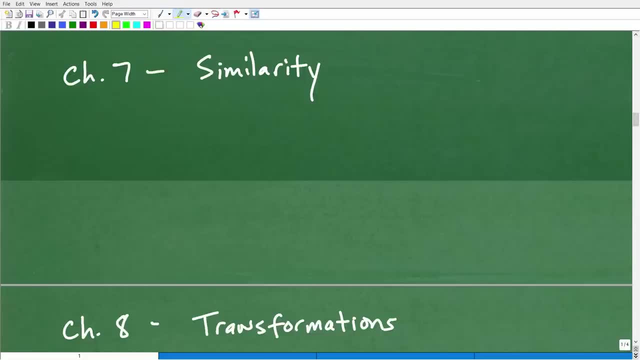 my thing is not working, but i'm not going to stop this video and make this over again, i'm just going to move on here. similarity, okay, so what is similarity? well, similarity is that one little squiggly figure right there. so let me just kind of show you that. so let's say i have a little. 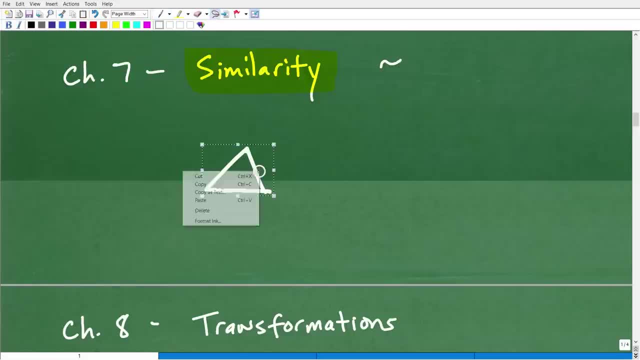 triangle like this, okay, and let's just uh kind of really make sure you understand. okay, so these two triangles together are exactly the same copy of one another. so these two triangles right here, this would be an example of congruence. that's what congruency or congruency is: it's an exact copy of one another. however, in this particular 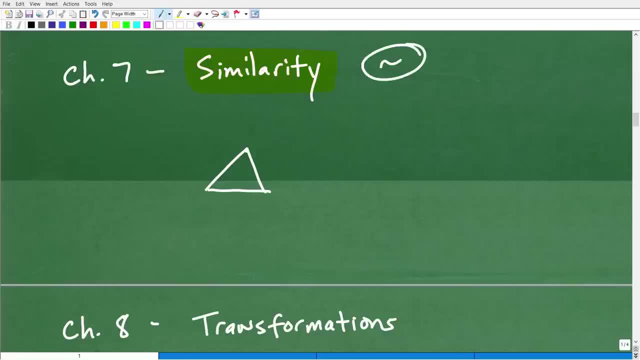 chapter going to be dealing with similarity, and similarity is a different deal, and similarity is kind of a zoomed in or zoomed out copy of that figure. okay, so if you are given one figure and you zoom in, or if you're given one little figure and you zoom out, okay, uh, vice versa, this. 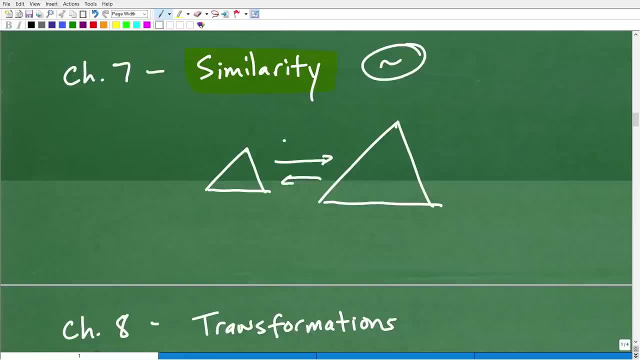 little figure and you zoom out, okay. vice versa, this is similarity, okay, so similar figures have the same angle measure, okay, and their sides, the respective sides, are in proportion, all right, so, uh, you're going to find out in this particular chapter. you're going to be setting up a lot of. 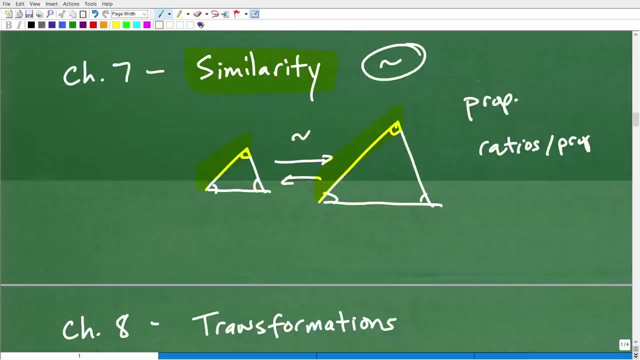 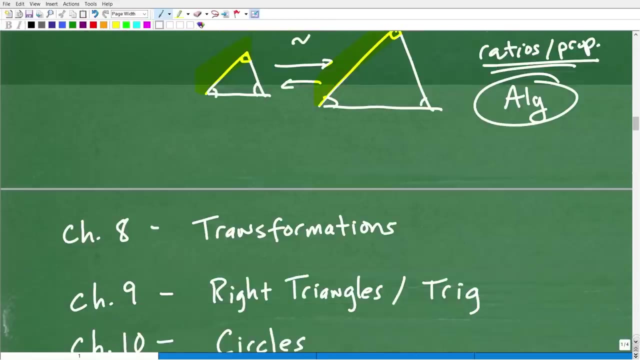 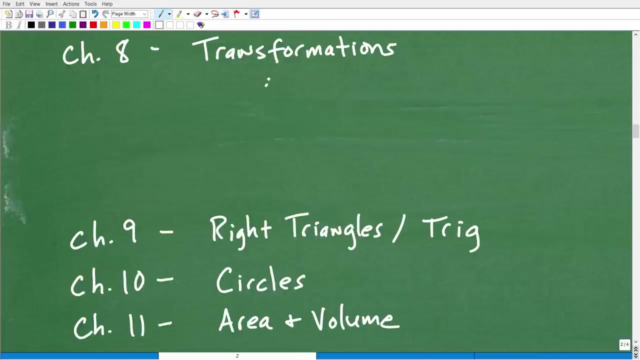 ratios and proportions to solve problems. okay, very, very important that you understand the difference between similarity and congruency and, again, ratios and proportions- things that you learned in algebra. okay, you're going to have to bring all your algebra skills to geometry for sure. okay, let's move on to our next thing here. oh, look at it, did it for me. 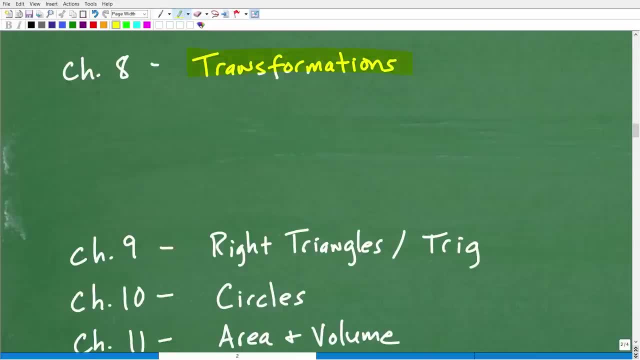 finally, i was able to space out and that is, uh, transformations. okay, so what am i talking about with transformations? well, transformations are basically- let me just show you this real quick- things that we can do with a figure. so let's say, i have a figure like this, okay, and i want to rotate. 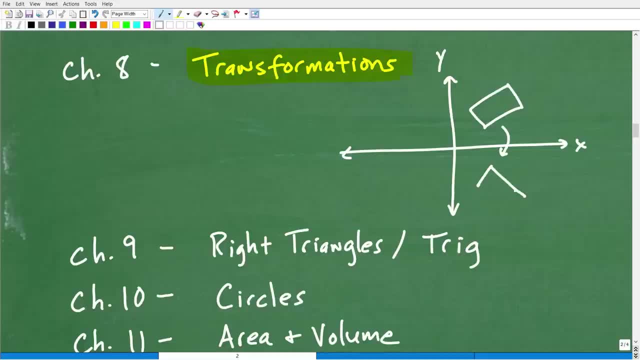 it. let's say i want to rotate it clockwise over here. that would be a transformation. or maybe i have a box right there and i flip it across the x-axis, it would be right there. so transformations are things like rotations. okay, uh, let's see here um. 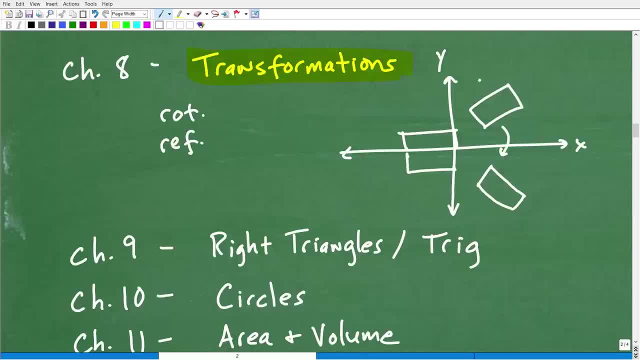 reflections. all right, if i could reflect something across the x-axis, this point reflected, its mirror image would be over here. so if this is point a, this would be like a prime, and so we have rotations reflections. we have these things called dilations, which are pretty cool. this is kind of. 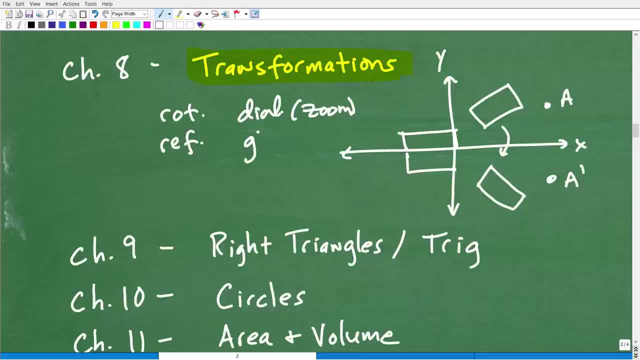 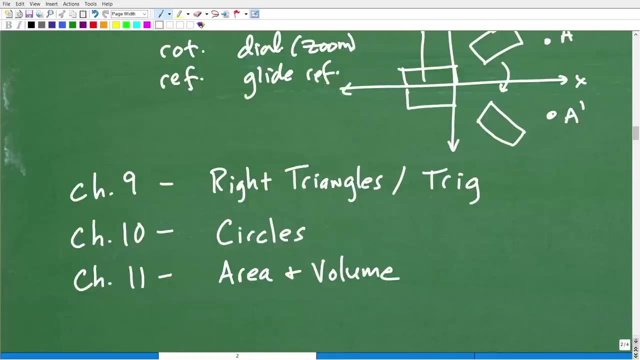 when you zoom in and out and then you think you have something called like glide reflections as well, okay. so, where you kind of take something, you move it up and then you shift it over to the right, but that's the whole idea behind, uh, transformations. okay, so again, you're going to have a whole chapter on that and we got three chapters. 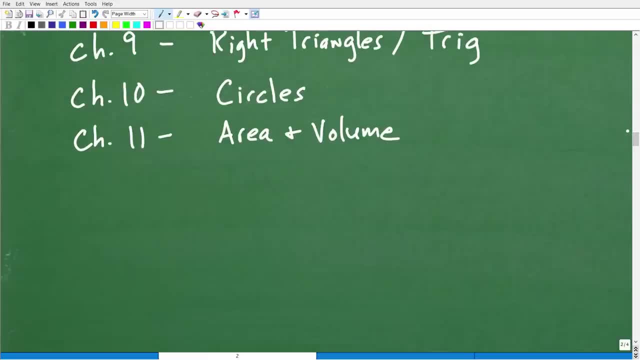 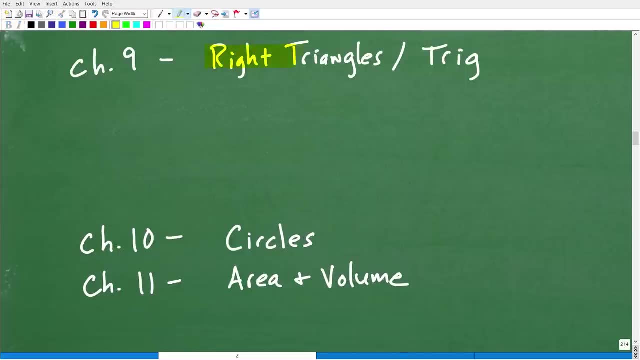 here. i probably went over 10 minutes, but hopefully you're still with me because you're interested in this stuff. okay, all right, so let's move on. and now we have right triangles and basic trigonometry. again, this is our third uh chapter that has to do with dedicated uh: two triangles. okay, so now we're. 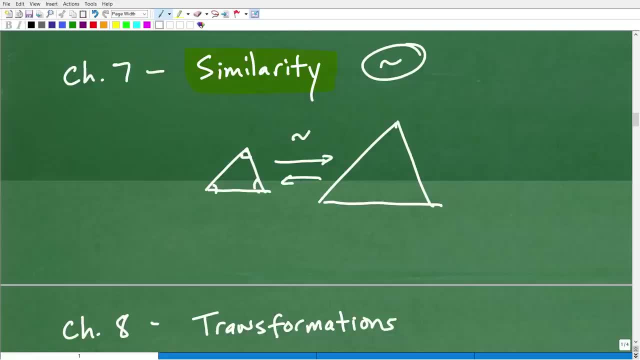 is similarity, okay, so similar figures have the same angle measure, okay, and their sides, the respective sides, are in proportion, all right. so, uh, you're going to find out in this particular chapter. you're going to be setting up a lot of ratios and proportions to solve problems. okay, very, very important that you understand. 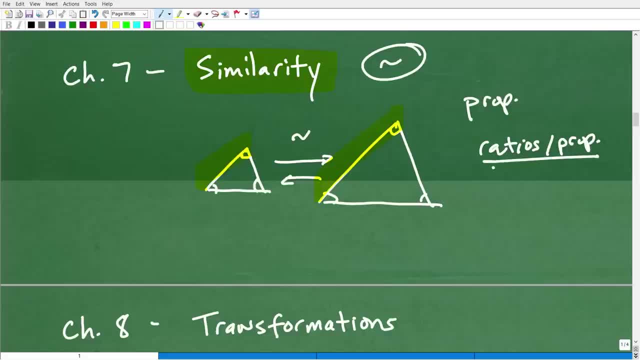 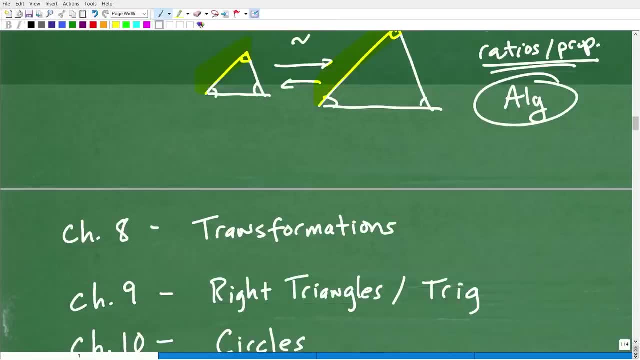 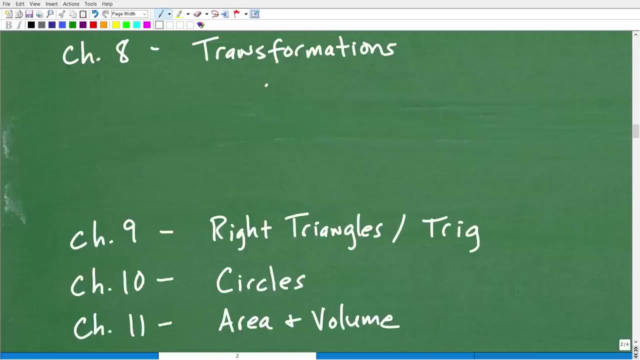 the difference between similarity and congruency, and again, uh, ratios and proportions- things that you learned in algebra. okay, you're gonna have to bring all your algebra skills to geometry for sure. okay, let's move on to our next thing here. oh, look, it did it for me. finally, 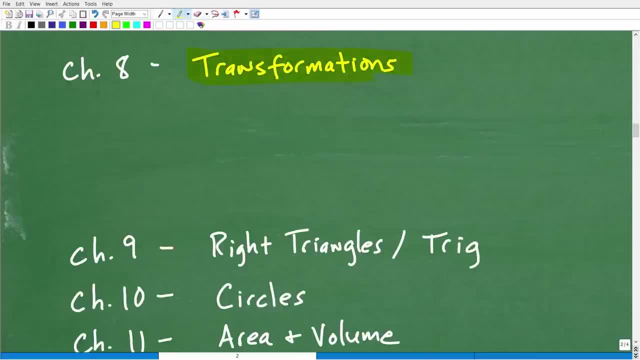 i was able to space out and that is, uh, transformations, okay, so what am i talking about with transformations? well, transformations are basically- let me just show you this real quick- things that we can do with a figure. so let's say, i have a figure like this, okay, and i want to rotate. 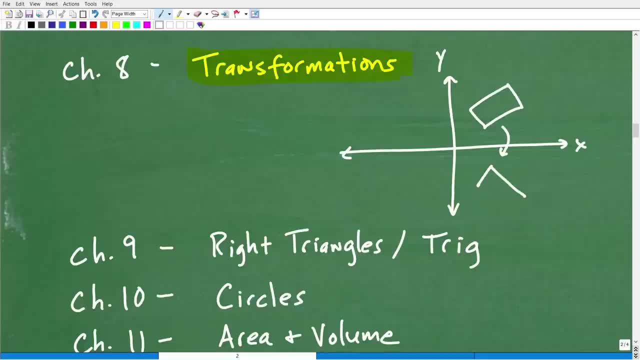 it. let's say i run over here and i want to rotate it and i want to rotate it and i want to rotate it and i wrote it rotated clockwise over here. that would be a transformation. or maybe i have a box right there and i flip it across the x-axis, it would be right there. so transformations are things. 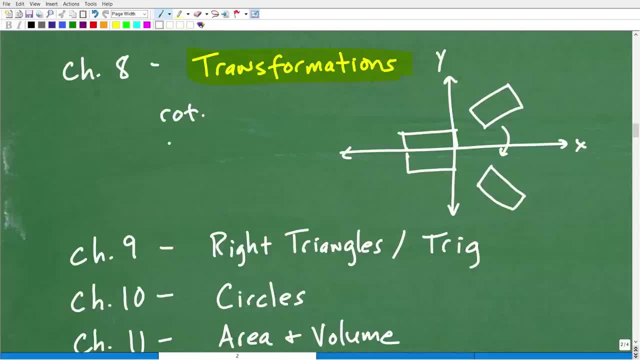 like rotations. okay, uh, let's see here, um, reflections. all right, if i could reflect something across x-axis, this point reflected, its mirror image would be over here. so if this is point a, this would be like a prime, and so we have, uh, multipleizing, right. so if i then rotate? 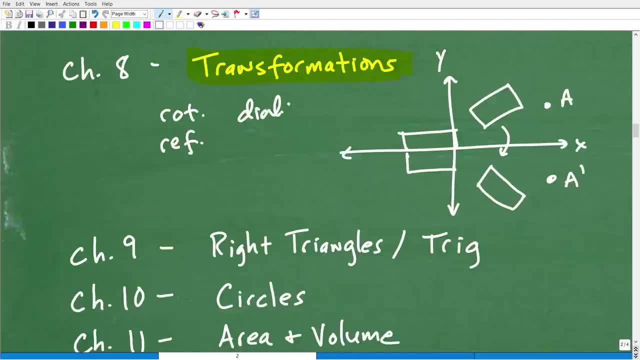 it and then if i flip it over here, the loss z deriving from is 0. but if i rotate this over here- locations, reflections- we have these things called dilations, which are pretty cool. this is kind of when you zoom in and out and then you think you have something called like glide reflections, as 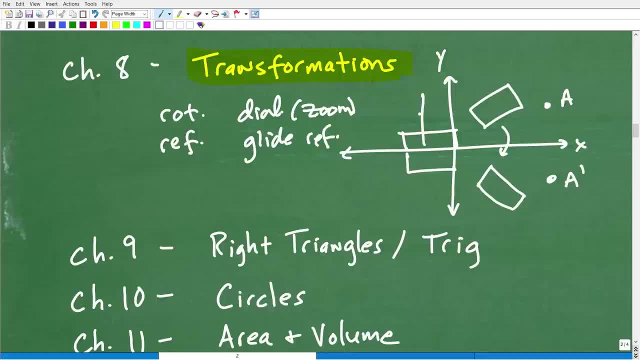 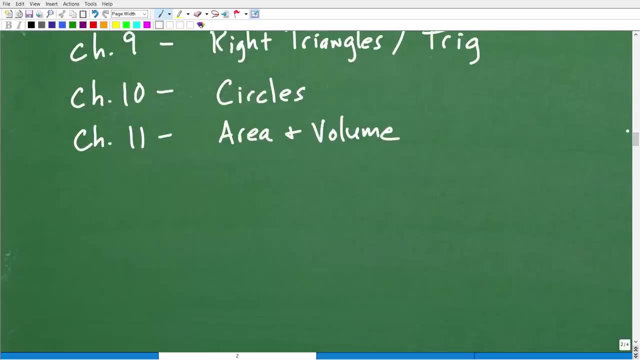 well, okay. so where you kind of take something, you move it up and then you shift it over to the right, but that's the whole idea behind, uh, transformations okay. so again, you're going to have a whole chapter on that and we got three chapters here. i probably went over 10 minutes, but hopefully you're still. 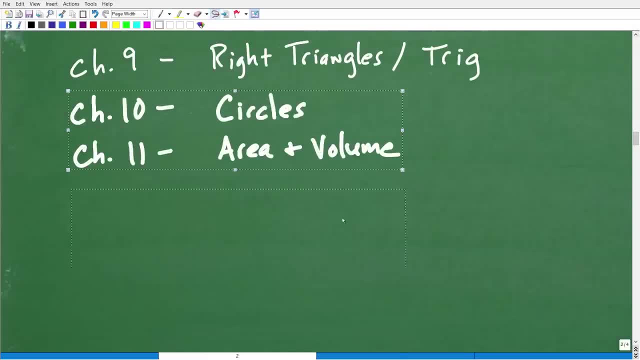 with me because you're interested in this stuff. okay, all right, so let's move on, and now we have right triangles and basic trigonometry again. this is our third uh chapter that has to do with dedicated uh. two triangles, okay. so now we're talking about right triangles again. that's where. 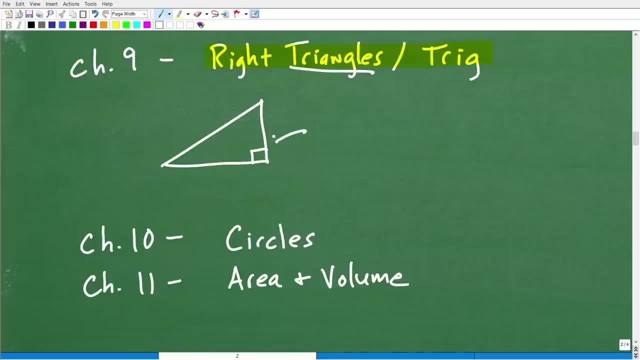 talking about right triangles again. that's where one of the angles is 90 degrees, uh, represented by this little uh notation right there. excuse me, boy, i have technical difficulties and i'm having issues with my voice, but guess what? that's not going to stop me. all right, let's move on and talk about. 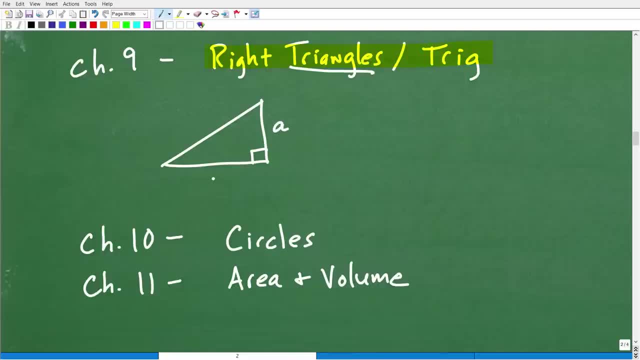 right triangles. so what are we talking about? some of the? what are some of the things we're going to be talking about in this chapter? we're going to be talking about, like the pythagorean theorem, a squared plus b squared is equal to c squared. definitely going to need to know how to deal with this, for sure you're also 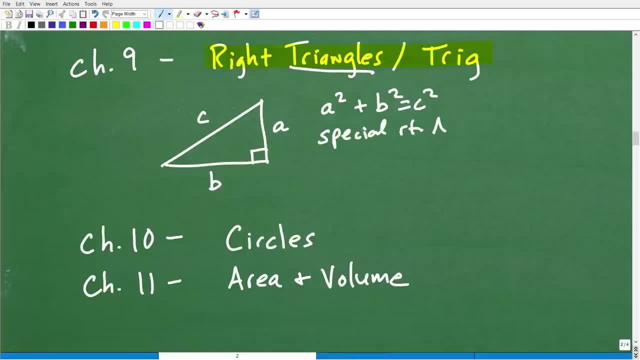 going to be talking about special right triangles. this is very important. so you're talking like 30, 60, 90 and 45, 45- 90 degree right triangles. now, in this chapter as well, you're going to learn basic trigonometry. this is your stuff, like sine, cosine and tan. 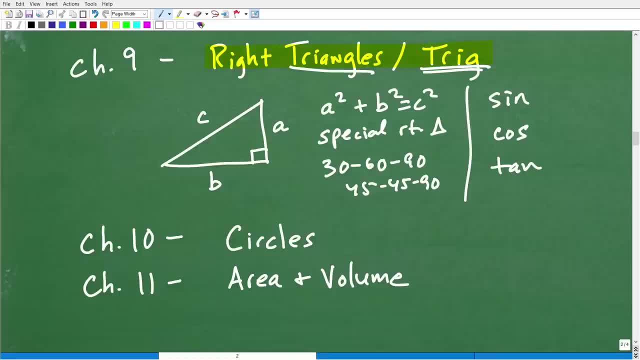 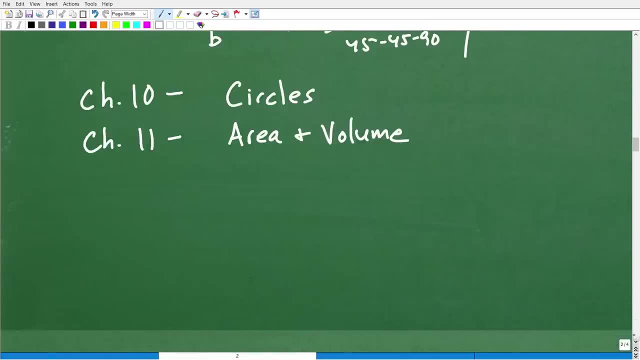 tangent very, very important, so you really get an introduction to trigonometry in this chapter as well. okay, so we're almost done and uh, you know, maybe i should do these video videos in advance time it. but you know, i just don't. you know, i just kind of go when i do videos. 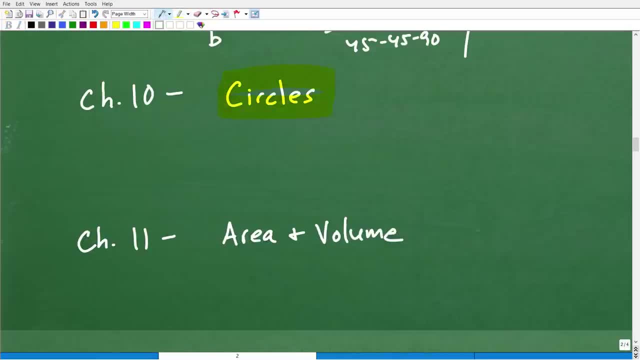 i make so many videos, i do the best estimation i can, but if i'm over 10 minutes please forgive me. but let's move on with our last two chapters. so chapter 10, in my course, is circles. okay, so what are we talking about with circles? well, obviously, uh, we're going to be talking about 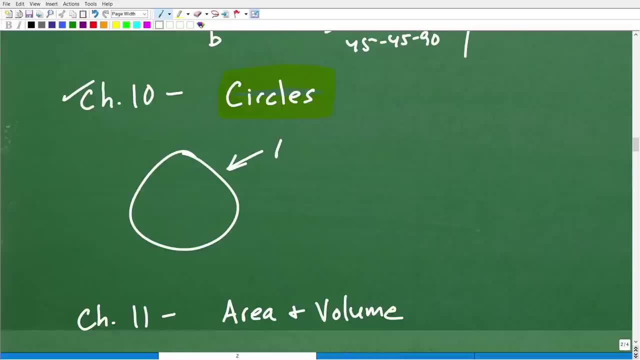 things that you already know. okay, so we have a circle, so you're going to learn about the area of a circle, the circumference of the circle, uh, basic, uh vocabulary about a circle like here's a diameter, there's a center, there's the radius, uh, all that kind of good stuff. 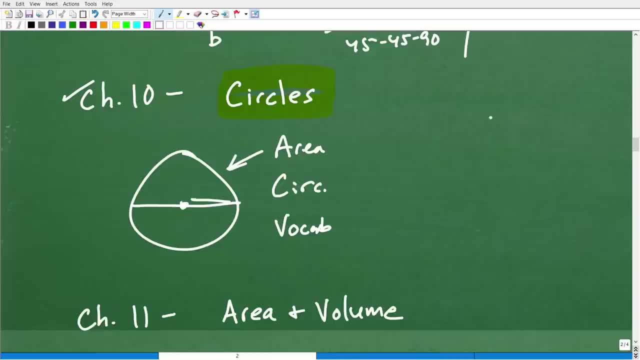 but you're actually going to be learning about different parts of a circle- very, very important as well. so we're going to be learning about things called a chord. okay, what happens if we have two lines that go through a circle? what happens to these angles and what happens. 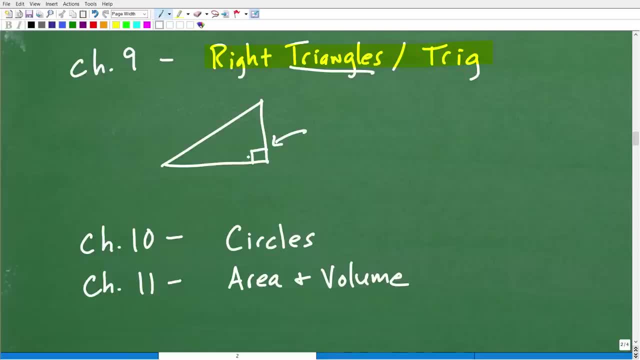 one of the angles is 90 degrees, uh, represented by this little uh notation right there. excuse me, boy, i have technical difficulties and i'm having issues with my voice, but guess what? that's not going to stop me. all right, let's move on and talk about right triangles. so 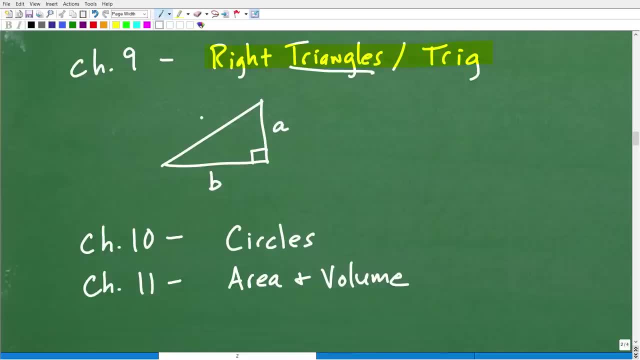 what are we talking about? some of the? uh, what are some of the things we're going to be talking about in this chapter? we're going to be talking about, like the pythagorean theorem, a squared plus b squared is equal to c squared. definitely going to need to know how to deal with this, for sure. 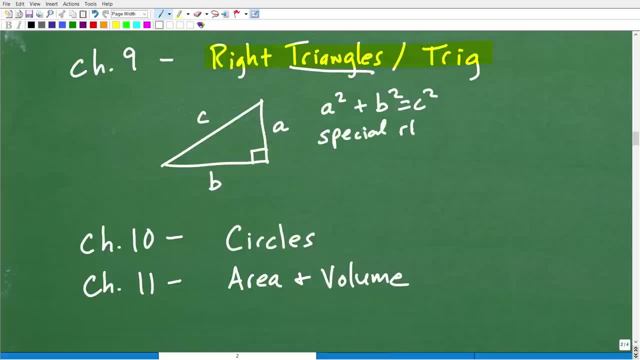 uh, you're also going to be talking about special right triangles. this is very important. so you're talking like 30, 60, 90 and 45- 45- 90 degree right triangles. now, in this chapter as well, you're going to learn basic trigonometry. this is your stuff, like sine. 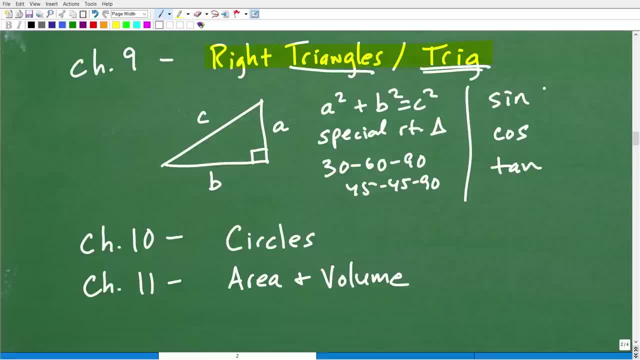 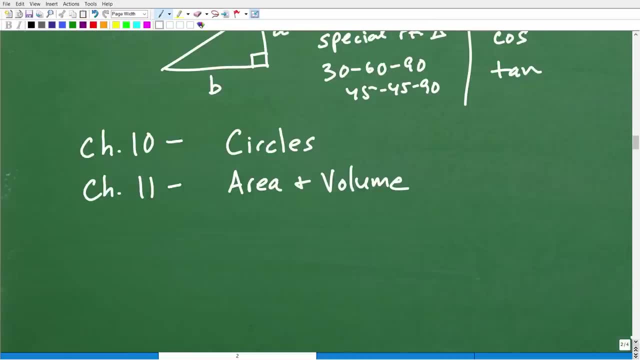 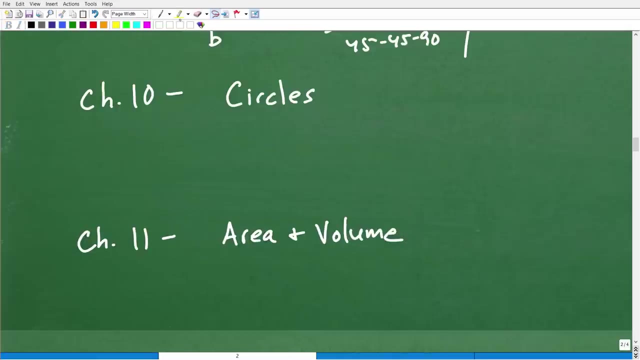 cosine and tangent very, very important. so you really get an introduction to trigonometry in this chapter as well. okay, so we're almost done and uh, you know, maybe i should do these video videos in advance time it. but you know, i just don't. you know, i just kind of go when i do videos. 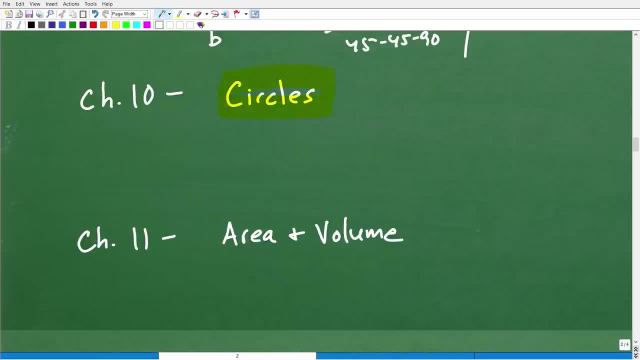 i make so many videos, i do the best estimation i can, but if you're interested in that kind of stuff. but if i'm over 10 minutes please forgive me. but let's move on with our last two chapters. so chapter 10, in my course, is circles. okay, so what are we talking about with circles? well, 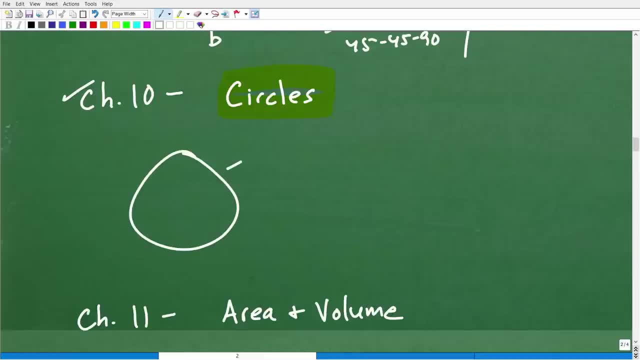 obviously, uh, we're going to be talking about things that you already know. okay, so we have a circle, so you're going to learn about the area of a circle, the circumference of the circle, uh basic vocabulary about a circle like: here's a diameter, there's the center, there's the radius, uh all that. 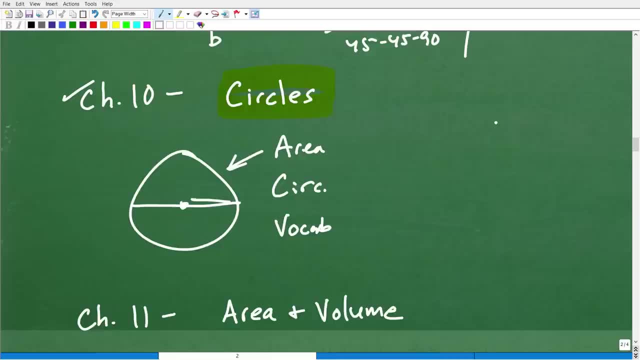 good stuff, but you're actually going to be learning about different parts of a circle- very, very important as well. so we're going to be learning about things called a chord. okay, what happens if we have two lines that go through a circle, what happens to these angles and what happens with 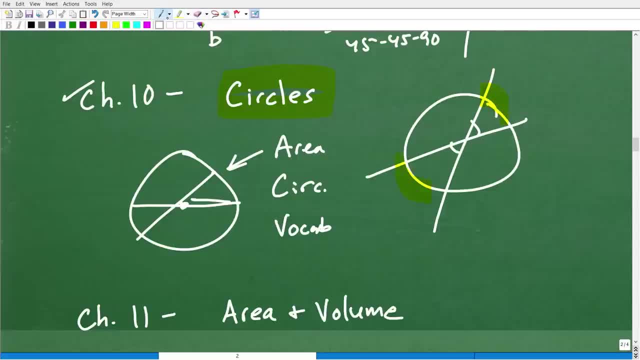 with these arcs in here. so there's a lot of different things you're going to need to know about inscribed angles. that would be something like this: okay, so if i have an angle inscribed inside of a circle, so what's the angle measure here if i'm given this arc right there? so you, 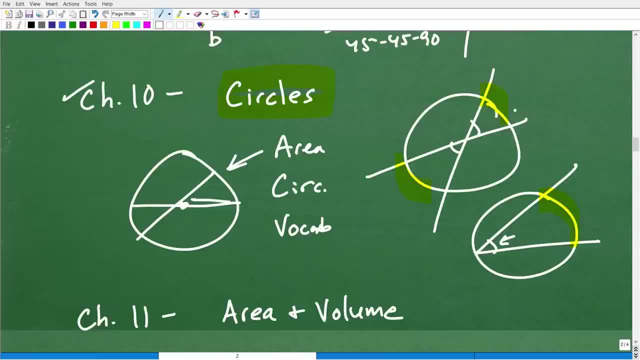 learned a lot of different properties and theorems- uh, about circles in this particular chapter. this is not that difficult. okay, again you're going to be doing some algebra work in here, but not heavy duty algebra as long as you need to. so as long as you know how to solve basic algebra, 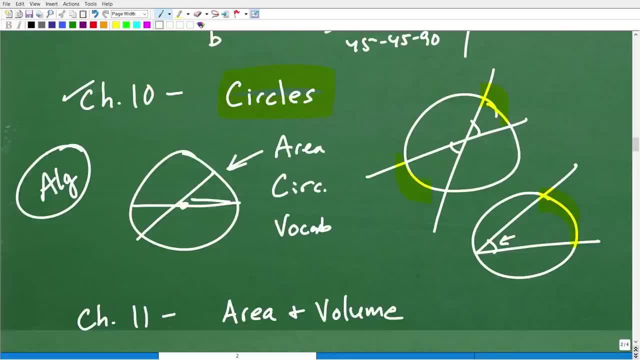 equations, you're going to be okay, but the whole thing here is just a lot of information. i don't think it's overly difficult. that's why you have to have super like awesome notes, very, very organized notes. there's way too much information given for you to remember. memorize all this stuff, okay, but 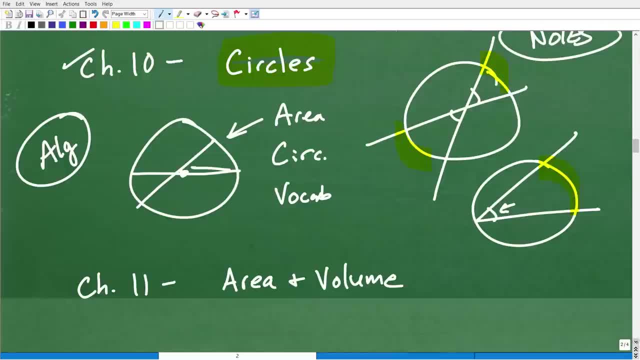 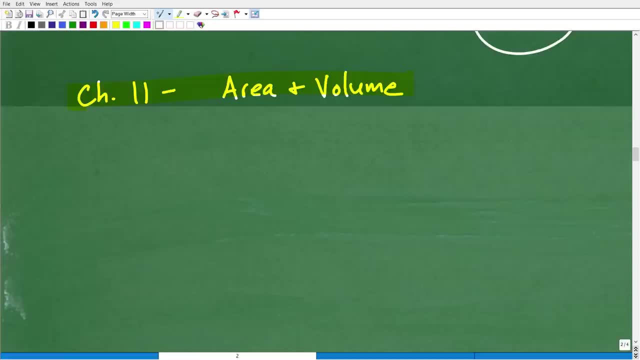 again, not difficult, just a lot of information. and finally, now let's go ahead and finish with this last chapter in my course, and that would be area and volume. so what are we talking about? well, we're talking about, uh, the area and volume of basic figures. so things like rectangles, squares, uh, circles, triangles, uh, trapezoids, uh. then we 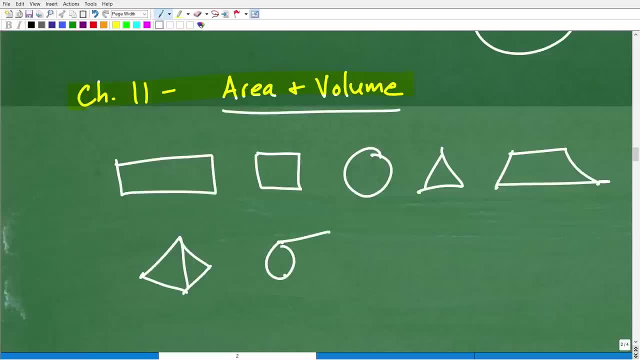 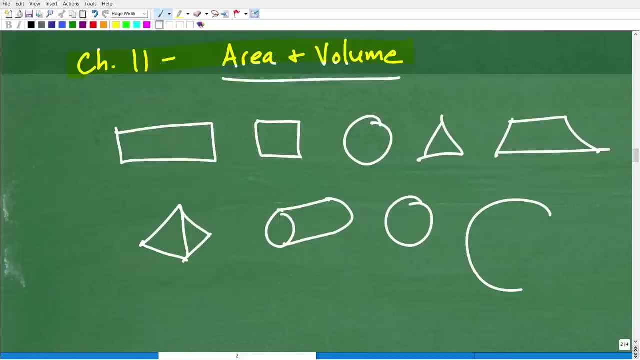 gotta get into like pyramids, uh, cylinders, okay, what more? we're talking about volume spheres and things that. uh, when we look at a circle, we could be talking about, uh, the area of like a little pi section here. okay, so that's a sector of a circle. okay, this is an arc and whatnot. so you really kind. 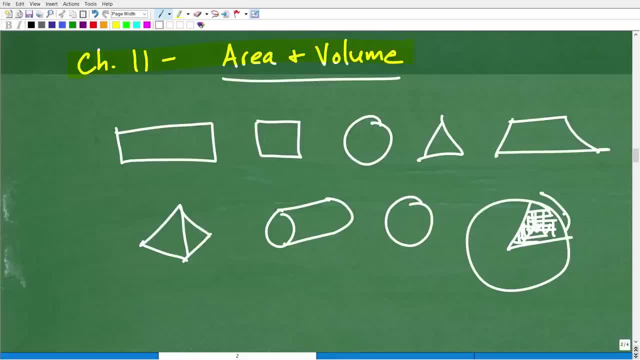 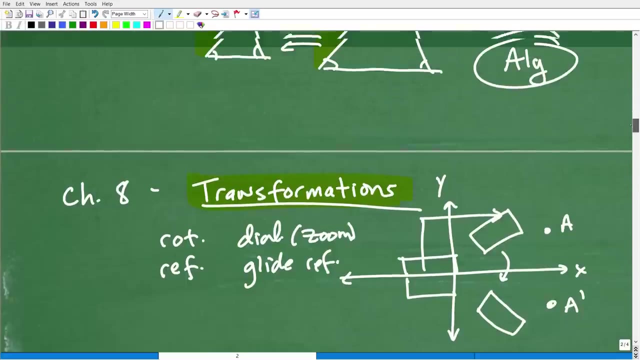 of get heavy duty into all. you know, we're talking about area, surface area, volume of all these basic figures, and then also sectors of circles as well, and this is it. uh, you know, probably went over 10 minutes. um, that's the case. so we might as well get started on this section, and i'd encourage you to take a look at this. 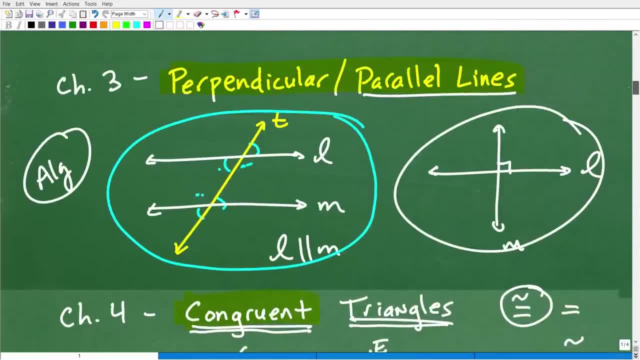 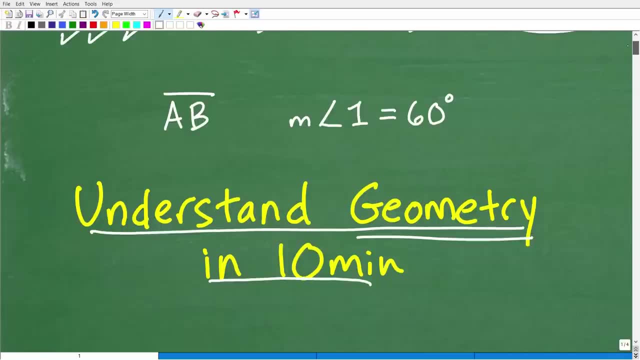 okay. so first let's have a look at some of our other videos. so we're talking about, uh, archaic geometries and you know i'm sorry for not being 100 perfect, but uh, you know, when you take a look at this, if you got a pretty good like, a basic sense of like, okay, i think i understand. 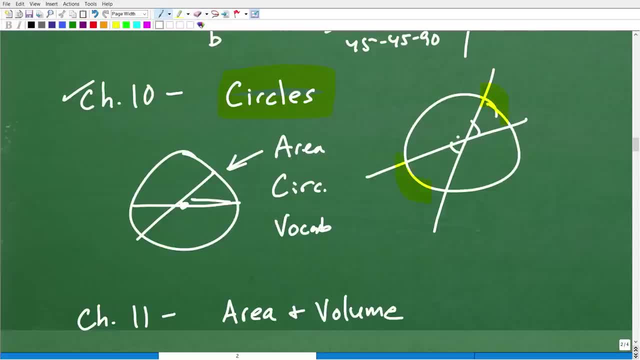 these arcs in here, so there's a lot of different things you're going to need to know about inscribed angles. that would be something like this: okay, so if i have an angle inscribed inside of a circle, so if i'm given this arc right there, so you learn a lot of different properties and theorems, uh, about 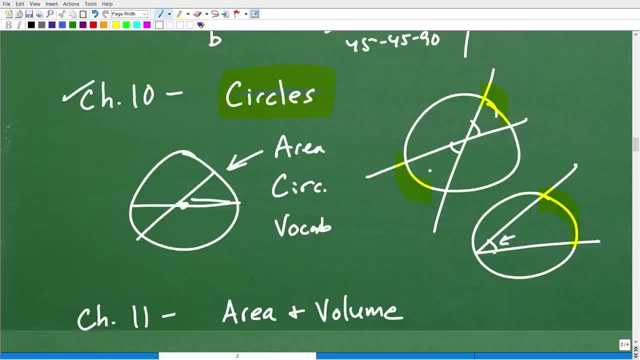 circles in this particular chapter. not, this is not that difficult. okay, again, you're going to be doing some algebra work in here, but not heavy duty algebra. as long as you need to, as long as you know how to solve basic algebra equations, you're going to be okay. but the whole thing here is just 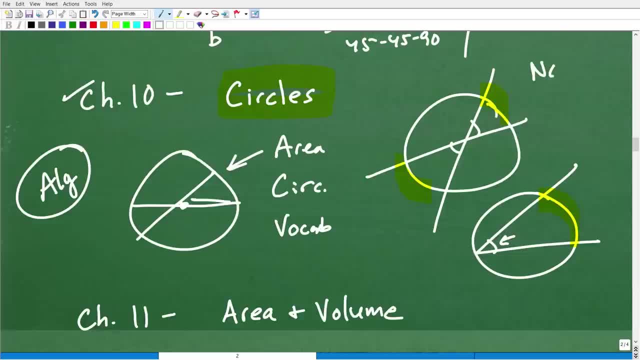 a lot of information. i don't think it's overly difficult. that's why you have to have super like awesome notes, very, very organized, and you're going to be learning a lot of different things and you're going to have super nice notes. there's way too much information given for you to remember. 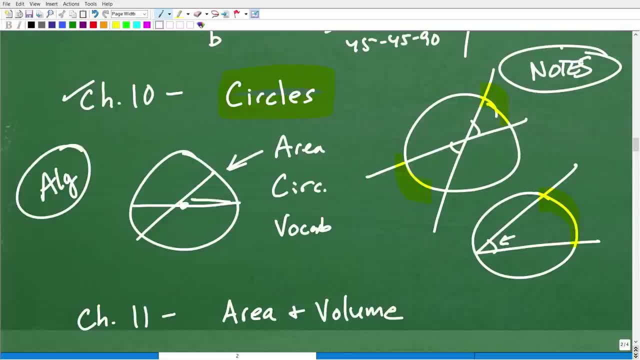 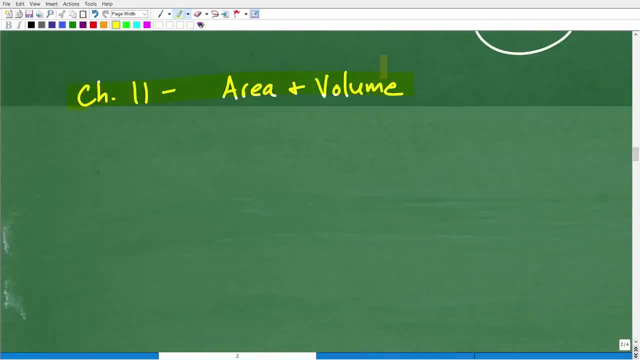 memorize all this stuff. okay, but again, not difficult, just a lot of information. and finally, now let's go ahead and finish with this last chapter in my course, and that would be area and volume. so what are we talking about? well, we're talking about the area and volume of basic figures. 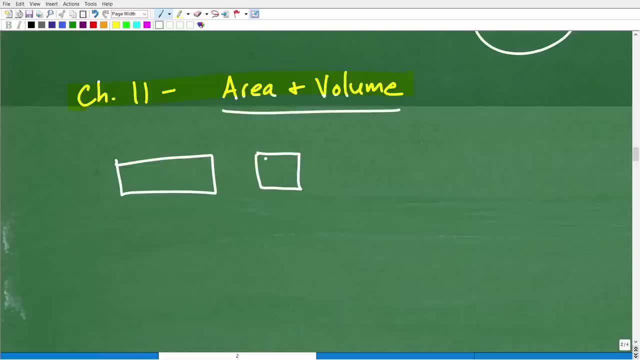 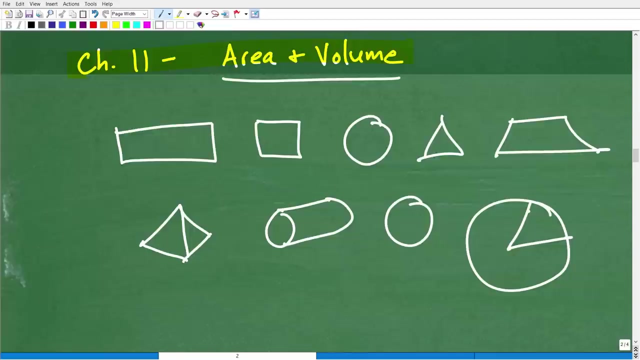 so things like rectangles, squares, circles, triangles, trapezoids, uh, then we can kind of get into like pyramids, uh cylinders, okay, when we're talking about volume spheres, and then uh things that uh, when we look at a circle, we could be talking about, uh, the area of like a little pi section here, okay. so that's a sector of a circle, okay, and this is an. 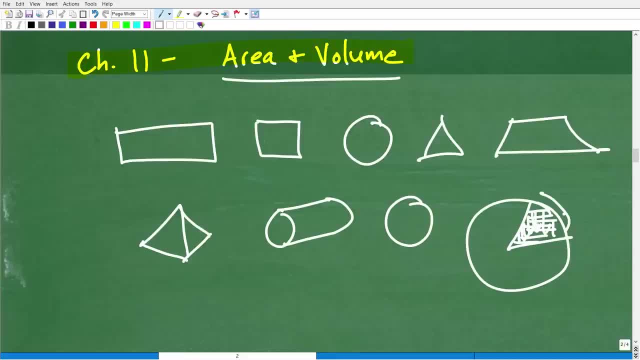 arc and whatnot. so you really kind of get heavy duty into all. you know, we're talking about area, surface area, volume of all these basic figures, and then you're going to be talking about the then, um, also sectors of circles as well, and this is it. uh, you know, probably went over 10 minutes. 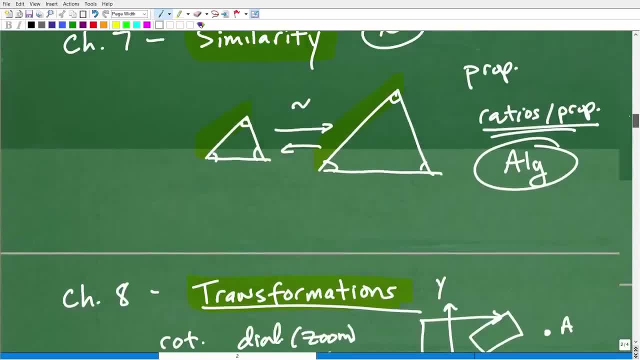 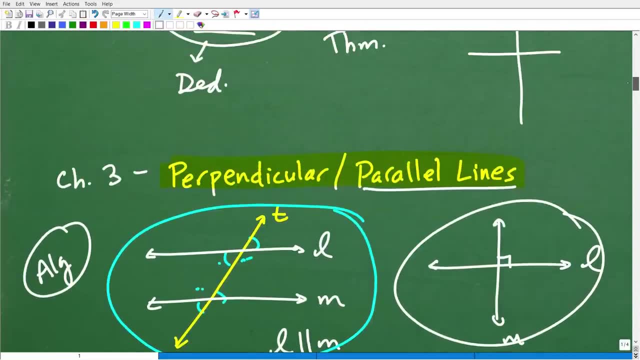 um, that's the case. you know i'm sorry for not being 100 perfect, but uh, you know, when you take a look at this, if you got a pretty good like, a basic sense of like, okay, i think i understand what are you saying, well, then you kind of have a pretty good feel, an overview of what you're.